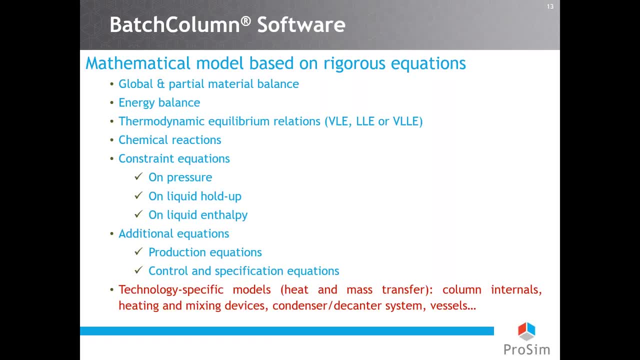 column for heat and mass transfer. For example, to accurately model the type of internals used in the column, heating and mixing devices, the condenser-decanter system and all the vessels which are associated to the column. This is very important to note that the dynamic 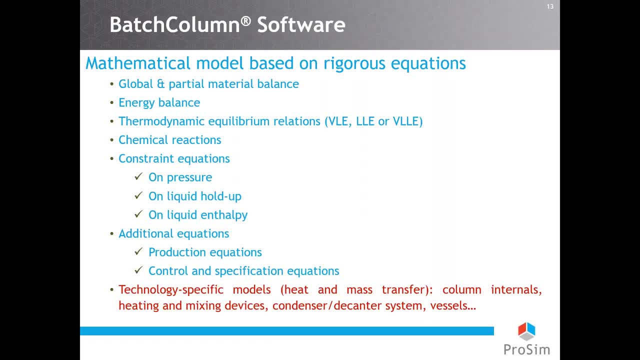 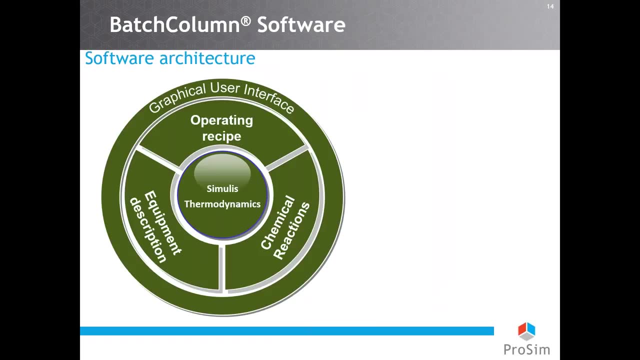 of the system is strongly linked with the technology, which has to be very precisely defined if we want to have accurate results. BatchColumn has a friendly user interface to describe the flowchart. BatchColumn has a friendly user interface to describe the flowchart. 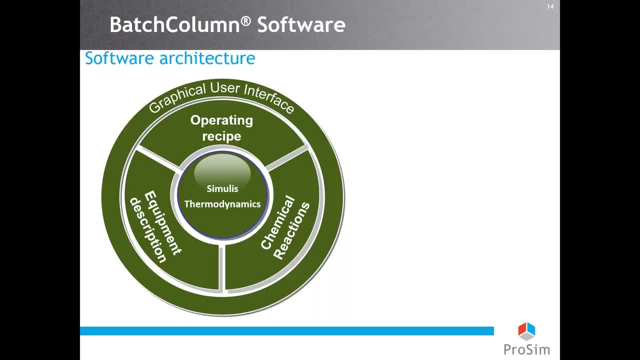 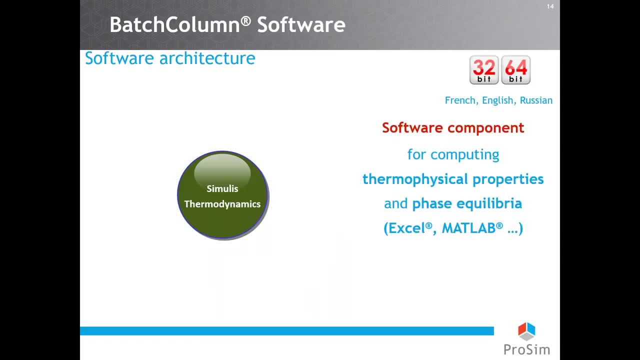 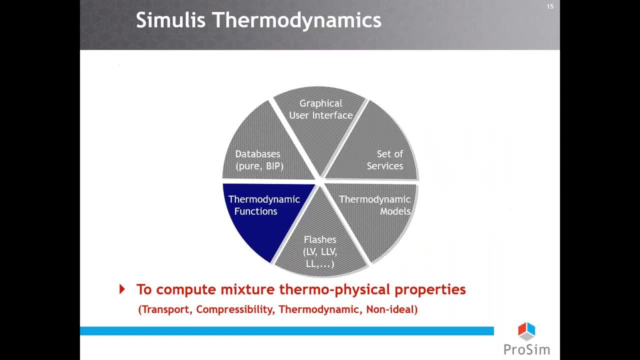 BatchColumn has a friendly user interface to describe the flowchart. The thermodynamics of batchColumn is unconditional thermodynamics, which is a software component to compute thermophysical properties and phase equilibria. BatchColumn is, understandably more than just the actual cool state. There are many pieces. 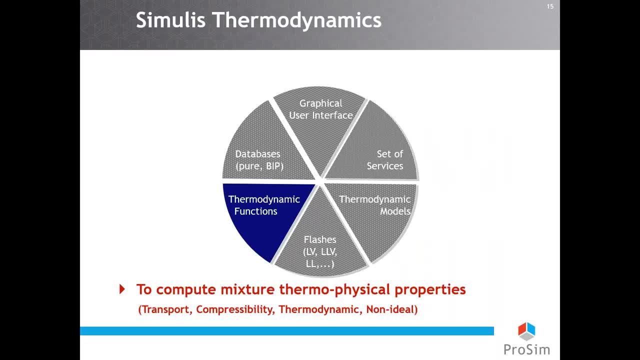 that make up this software component, which can be used to compute mature thermophysical properties such as transport compressibility. In addition to calculating the thermoic functions, the software uses temperature, pressure and overall composition to compute and to determine the phases which are present in the mixtures. 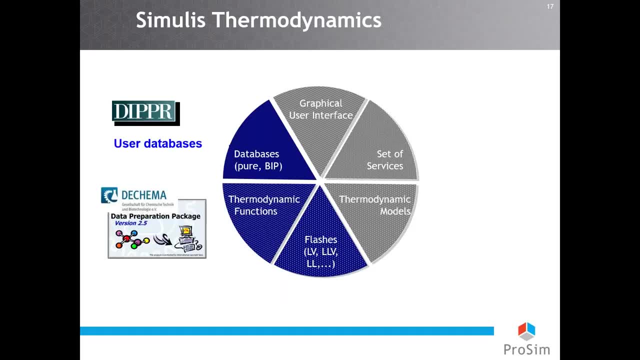 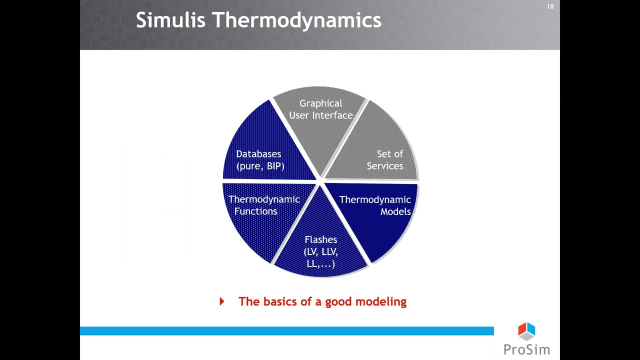 These are the FLASH calculations. In addition to these calculations, Simulacro Dynamics includes various databases that contain information required for mixture calculations, in particular databases for pure component properties and databases for binary interaction parameters. The thermodynamic model part is the main part of the system, of course, and the basis for 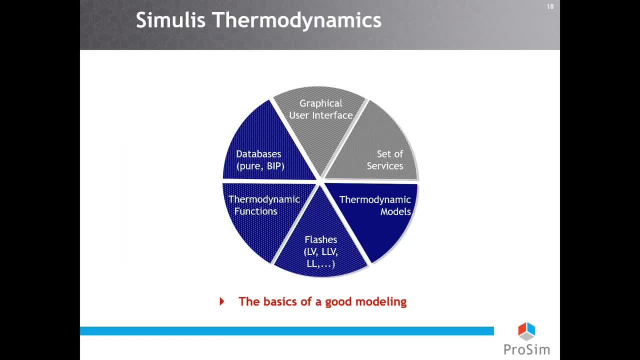 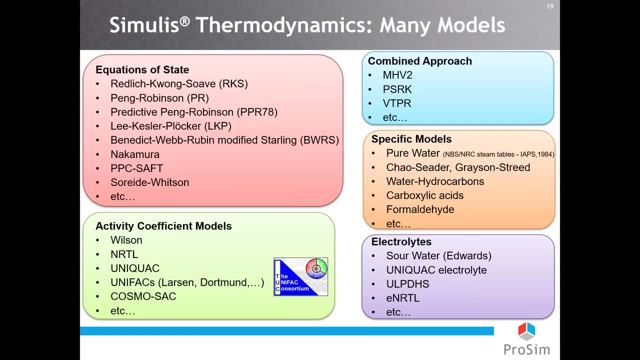 an accurate simulation for any distillation. Everybody knows that all models are wrong, but of course some are useful. The choice of a thermodynamic model depends on several things: The mixture you are working with. the temperature and the pressure conditions. the composition. 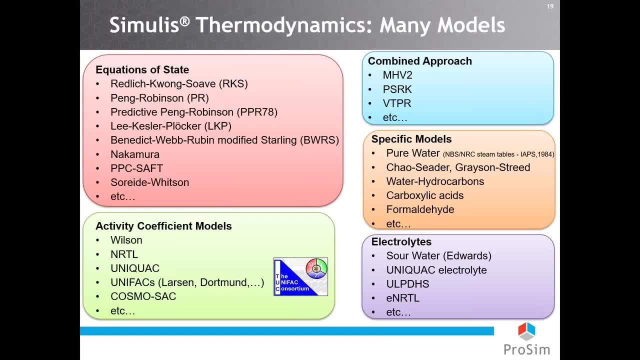 and so on. So to be able to address all of the different possibilities encountered in a process-insuring field, there are a lot of thermodynamic models available in Simulacro Dynamics. Its model library contains the most important thermodynamic models, including equation of: 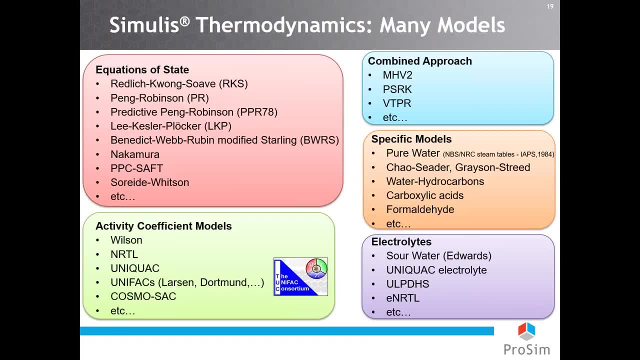 states, such as Redisch-Kong-Suave, Pang-Robinson or more sophisticated equation of state like the SAFT-based equation of state. We also have activity coefficient models such as the well-known NRTL, UNIQUAC or predictive. 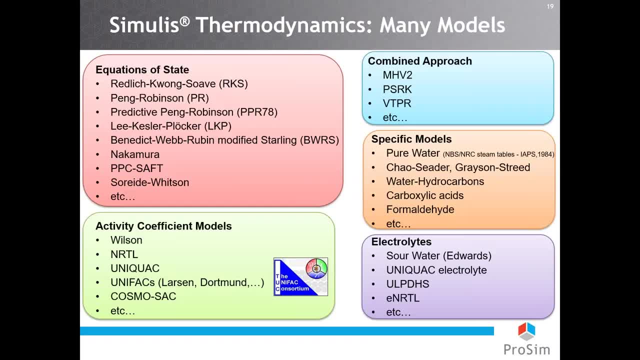 methods like UNIFAX or MORAL-FACTS. Thank you. You can also use what we call combined models. that means equation of state approach using complex mixing rules which include an activity coefficient model like the MHV-2, PSRK or. 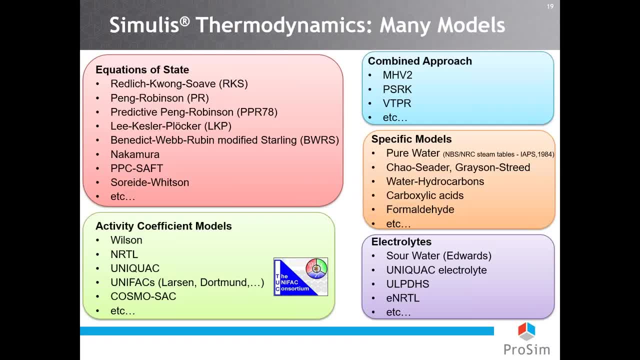 VTPR mixing rule. We also have some specific models, mainly for associating components, such as models for pure water or steam, for carboxylic acid and so on, and also some electrolytes models. Thank you, Thank you. 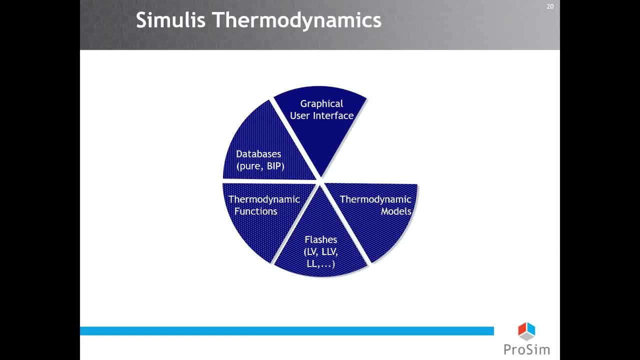 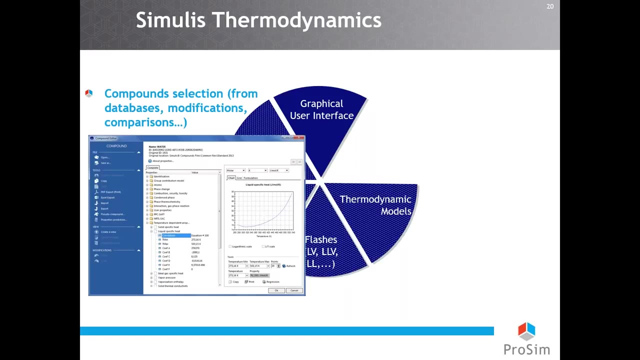 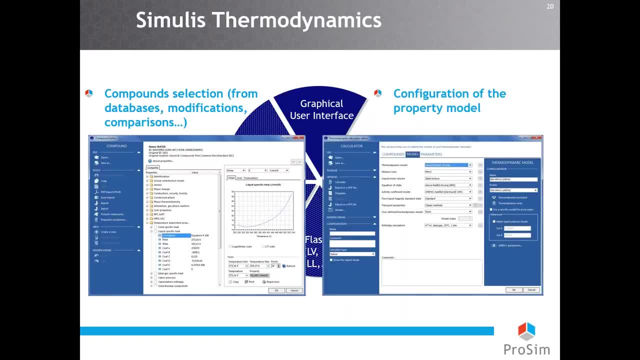 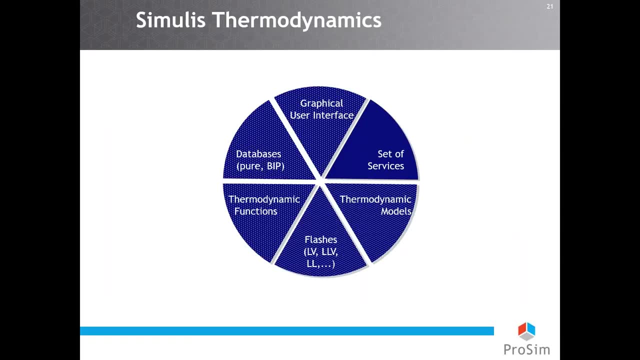 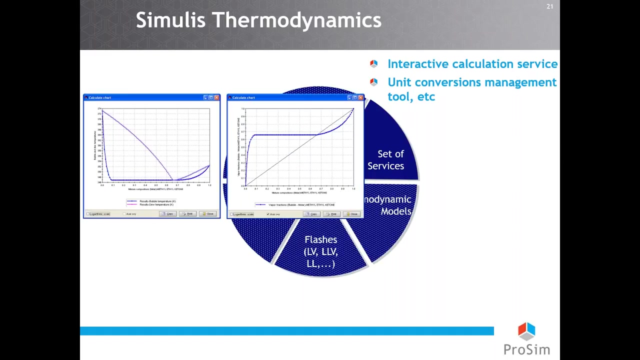 then also to choose and configure the appropriate mixture, thermodynamics and property models. Okay, Okay, The final piece of the software is the set of services that are included, such as the Interactive Calculation Service and the Unit Conversion Management Tool. The Interactive Calculation Service provides a user-friendly interface to quickly do all sorts of equilibrium and mixture property calculations. 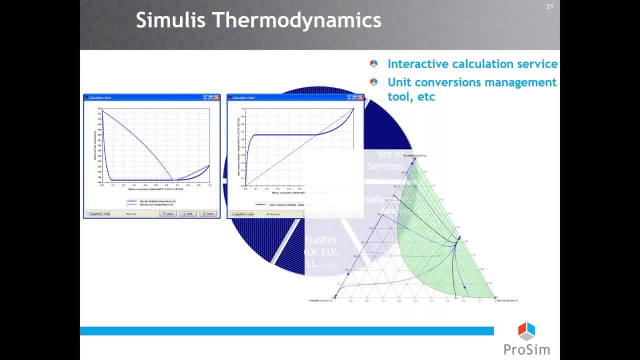 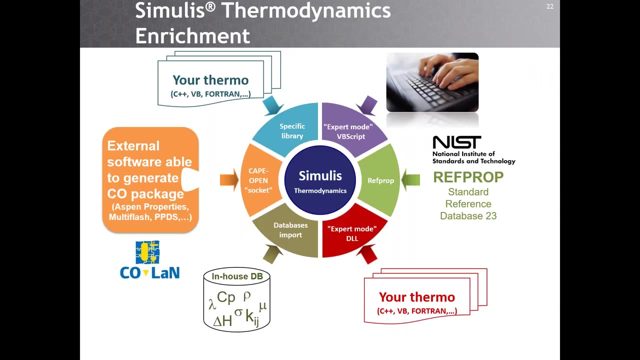 such as free-phase equilibria or, what is very useful when we are doing some distillation, residual curve map analysis. Simulist Thermodynamics can be also enriched. The user can import his own databases. Semantic packages from external software able to generate tape-open packages can be used, for example, coming from Aspen or MultiFlash. 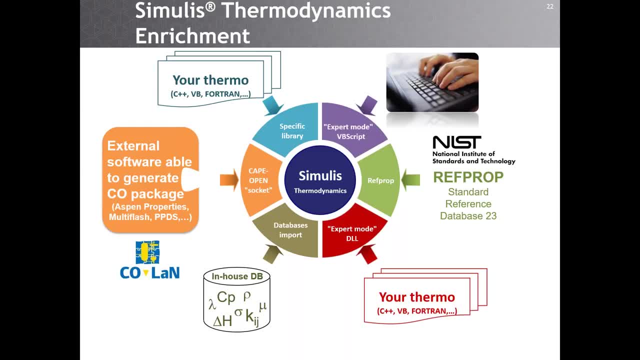 Procine can develop some specific libraries for its customers. For example, Air Liquide has its own model for air distillation included inside Simulist Thermodynamics. The user can also implement his own thermodynamic model very easily using the VBScript language. Thanks to the expert model, it can be used, for example, to represent the viscosity of a mixture using a simple model like a polynomial expression. 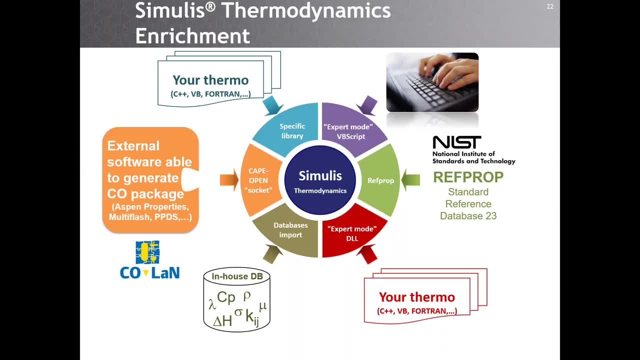 The user can also develop his own thermodynamic model using language such as Fortran, C++ or C Sharp. This can be very useful to use in-house thermodynamic code or to implement a new activity coefficient model or a question of state. In that case, native flashes of Simulist Thermodynamics can be used. 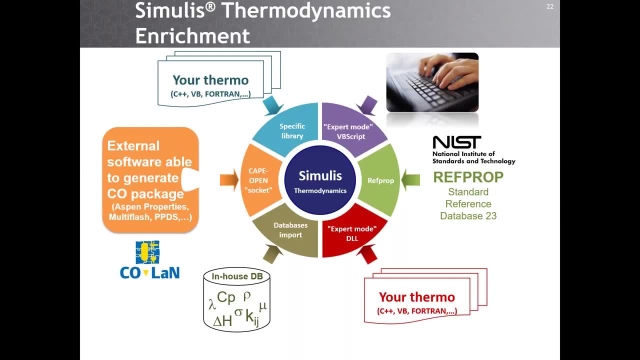 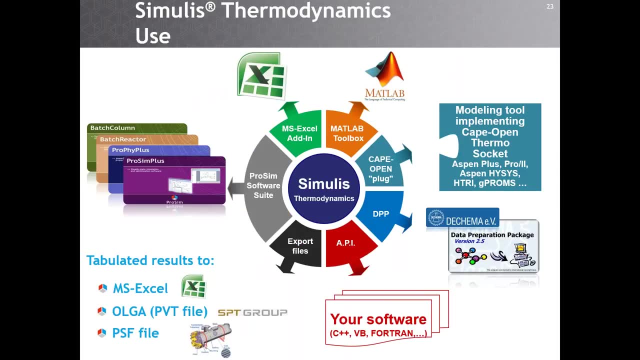 Simulist Thermodynamics also offers a source of information. Simulist Thermodynamics can be used as a socket to connect RevCrop to Simulist Thermodynamics. Thanks to its software component approach, the same software can be used in all environments used by chemical engineers. 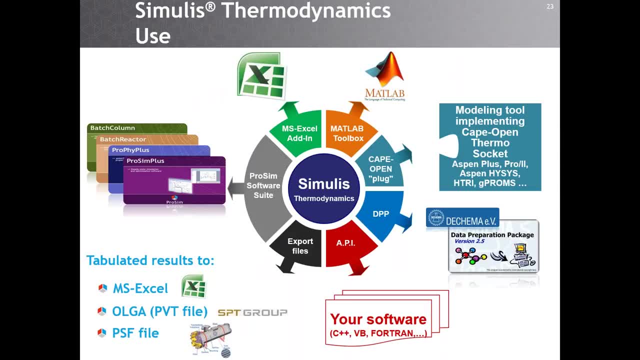 That means that users will have access to the same graphical user interface to describe his thermodynamic models, And it will be ensured that results will always be consistent between these environments. Of course, Simulist Thermodynamics is the thermodynamic earth of all Procine software. 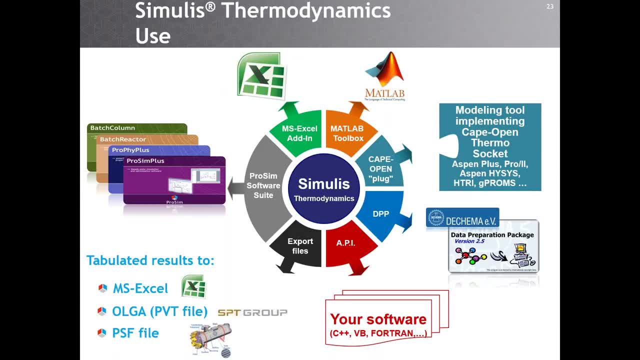 Simulist Thermodynamics is also available as an IDE in Microsoft Excel and as a toolbox in MATLAB. Thanks to the CapeOpen plug facility, one can use Simulist Thermodynamics package in CapeOpen software such as Aspen Plus Pro2, Aspen Isis and so on. 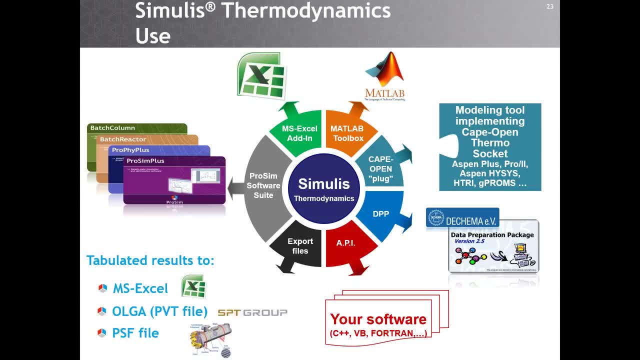 Users can use Simulist Thermodynamics within the software data preparation package from the Dekema to fit thermodynamic model parameters. Simulist Thermodynamics is also provided with the Dekema application. Simulist Thermodynamics is also provided with the Dekema application programming interface, an API which can be used to plug Simulist Thermodynamics in your in-house software. 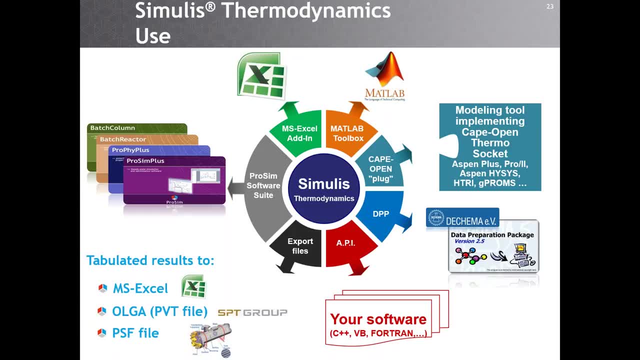 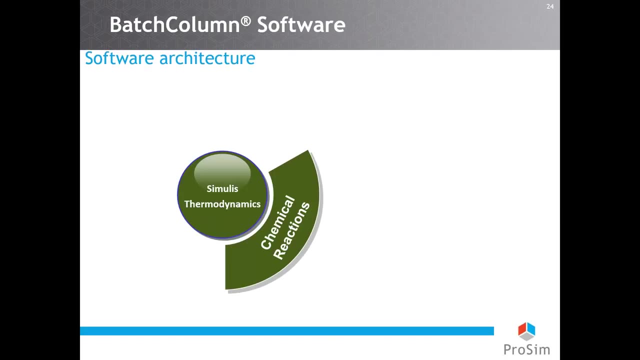 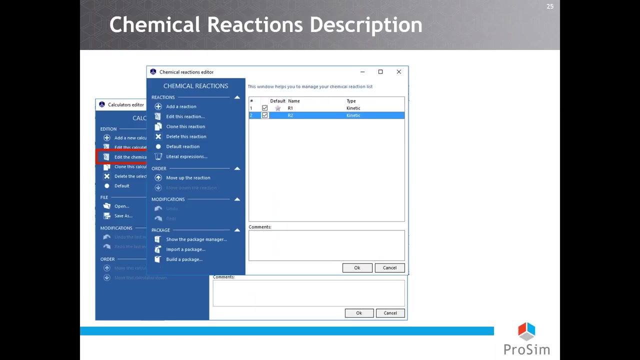 Calculation code, but also graphical interfaces and services are of course accessible, And you can also export Thermodynamics calculation results as tabulation results. If we come back to the batch column architecture, after the thermodynamic description one can describe some chemical reactions. Chemical reactions are associated to the thermodynamic calculator. 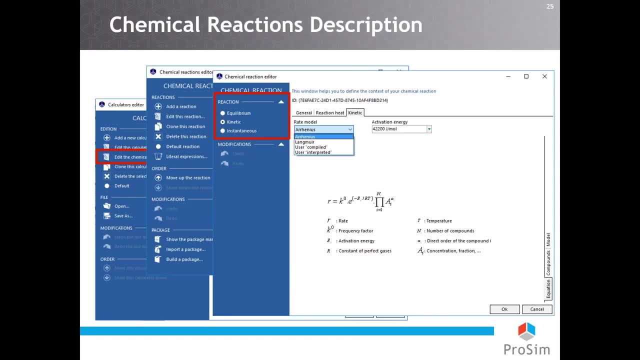 So you can describe the reaction scheme using different types of reactions: Equibrium reactions or reactions with a kinetic model. All the parameters are available to the user. Arrhenius and Langmuir formalisms are available to describe kinetic reactions. User can also implement his own model using VBScript option available inside the ThermoMirror. 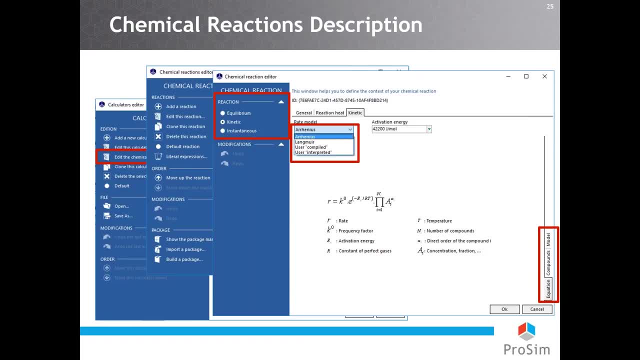 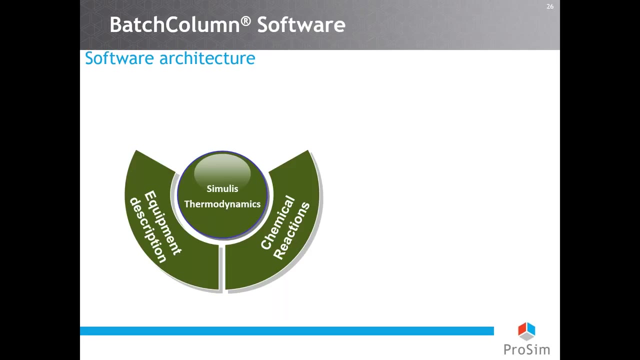 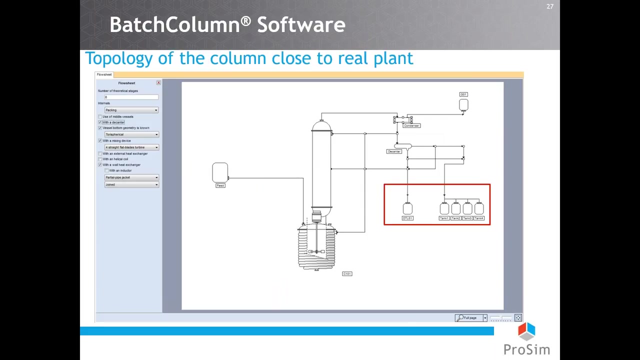 Or using an external DLL generated with any programming language. So, to conclude, there is no limitation regarding the reaction models. If we still coming back to the architecture of the software, now let's go to the equipment description, So you can describe as many fields of production tank as you want. 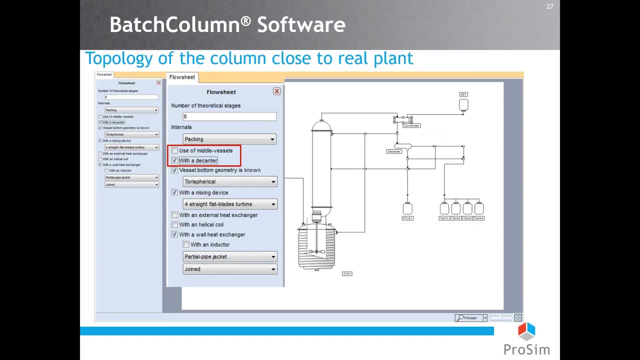 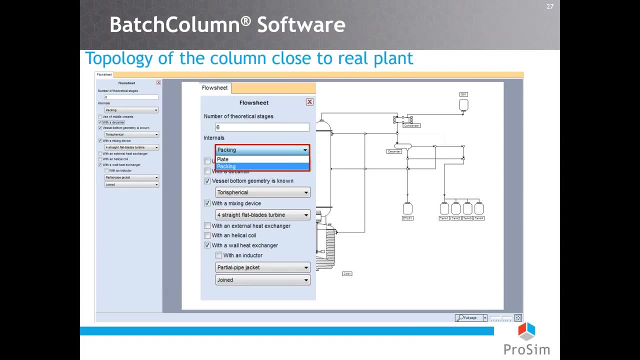 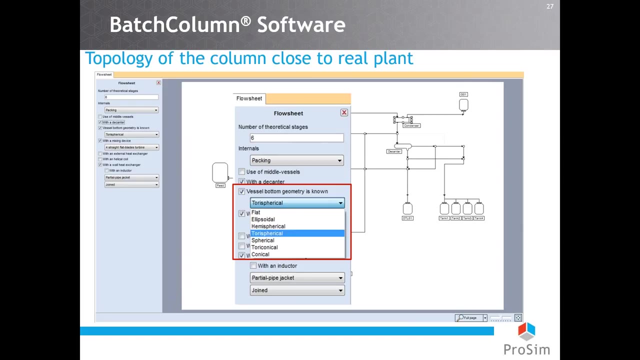 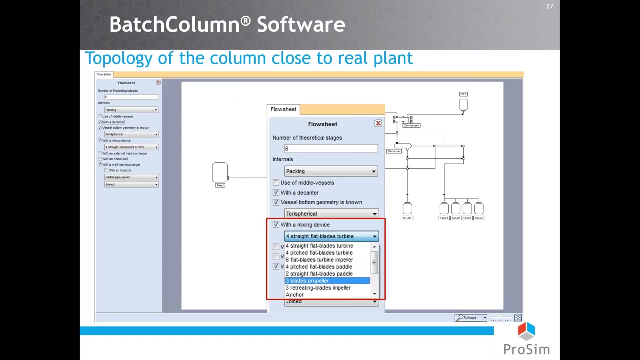 You can have column with the production tank. You can have column with the middle vessels with a decanter You can select the internals. You can have plate or packing internals. You can describe the vessel bottom geometry, if you know it. You can select the mixing device in a very large library. 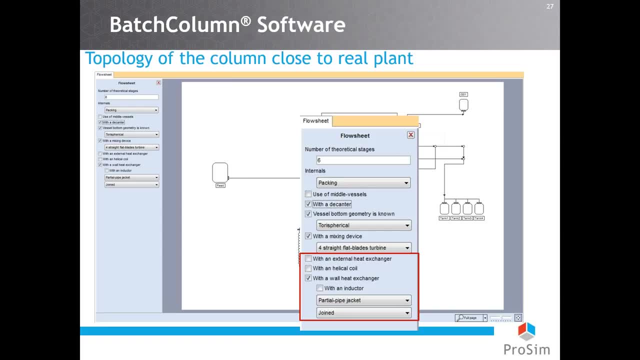 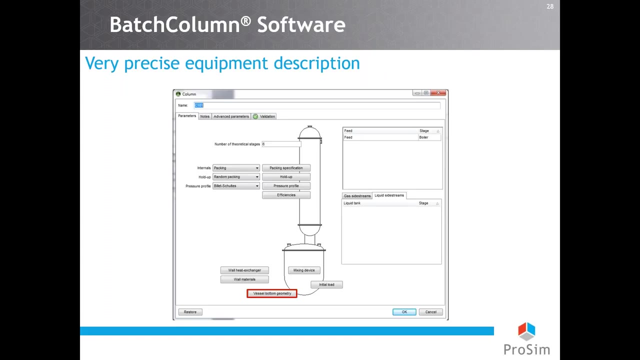 Regarding the heat exchange facilities, you have different kind, like external heat exchange or wood heat exchanger, And then you will, for each of these parameters, provide, for example, for the vessel bottom geometry. you will select what is the type of the vessel bottom geometry. 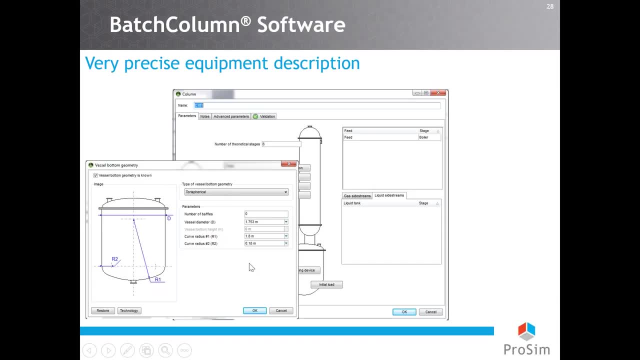 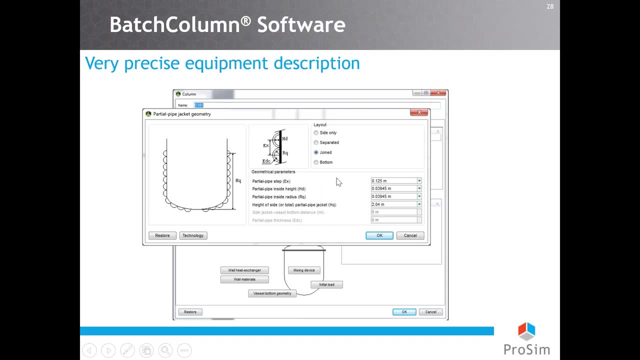 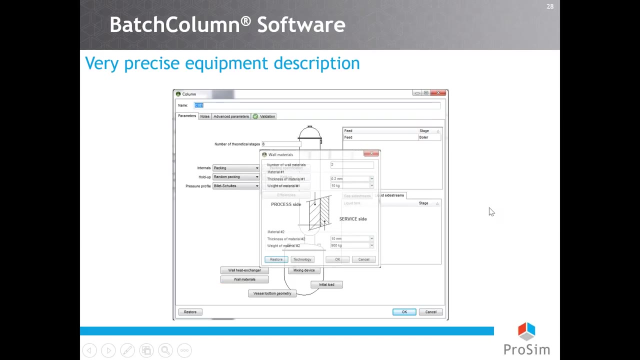 and then provide the corresponding parameters For the wood heat exchanger. you will also select what is the geometry you have and the corresponding parameters. Regarding the wool materials, you can describe just one material or two materials, For example, to represent glass line reactors. 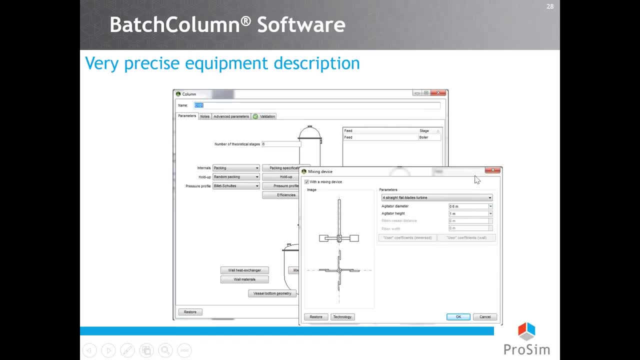 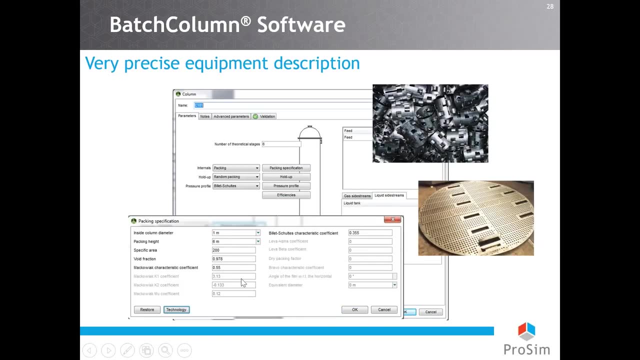 For the mixing device, you select it from the library and you provide the parameters, And for the internals, you will find also some library of internals for each material, For the packing or plate devices And regarding the condenser, you can describe with the real geometry. 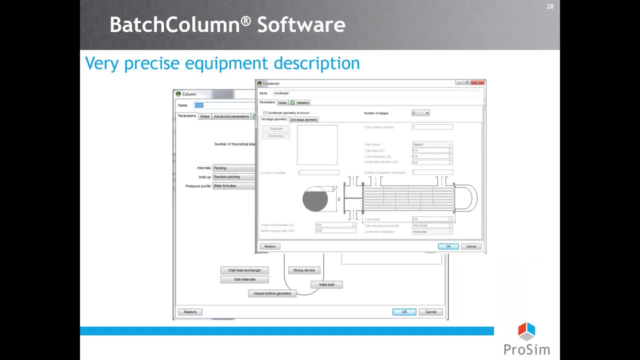 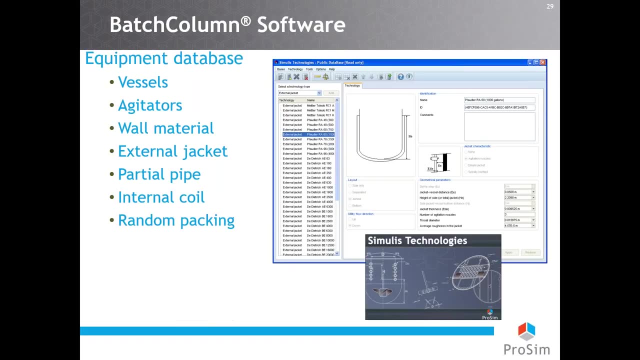 of shell and tube heat exchangers And you can have one stage or two stages for the condenser. Simulis Technologies is provided with BatchColumn. This software is used to manage equipment databases. BatchColumn includes standard databases for vessels agitators. 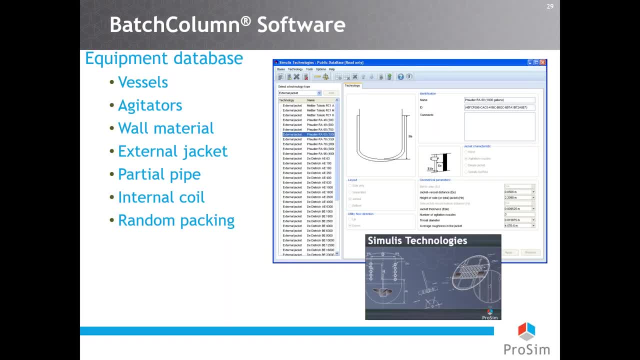 wool materials, external jackets, partial pipes, internal coils and random packing Characteristics stored in the database are coming from equipment manufacturers And, of course, users can also create their own private databases that contain exact descriptions of their own equipment. The last part of BatchColumn. 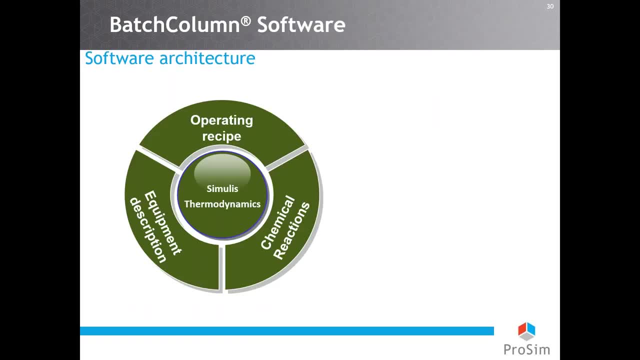 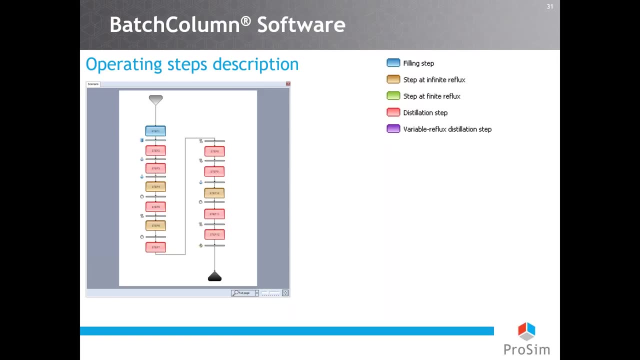 is the operating recipe description. After the characteristics of the column and the other device parameters are supplied, the user creates the production recipe, or what we call the scenario. A scenario is made of several steps. Each of these steps consists of specific operating conditions and stop criteria. 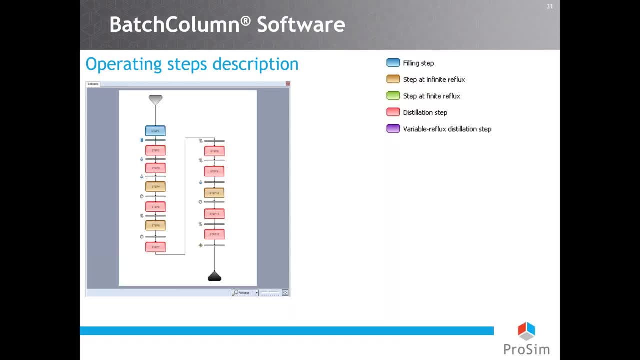 which are called events. Several predefined types of operating steps are available in BatchColumn. The filling step is used for the calculation of the boiler operating time And the filling time for all stages up to the commencer. A step at infinite reflux is used if the distillate is sent back. 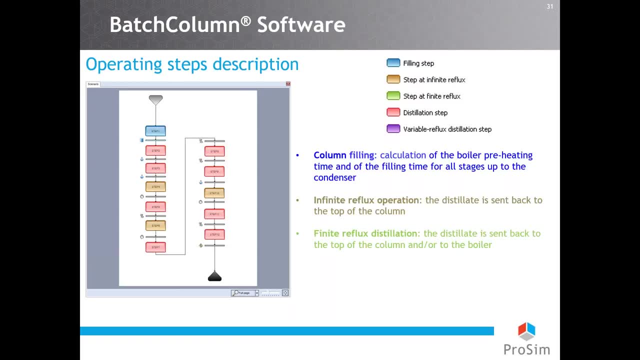 to the top of the column And a step at finite reflux is used if the distillate is sent back to the top of the column and out to the reboiler. And there are two distillation steps which are also available: One with a given reflux ratio. 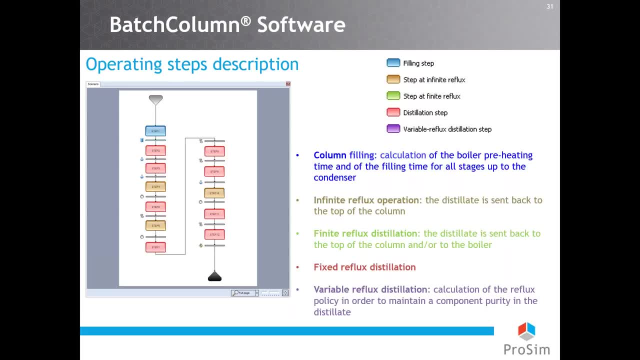 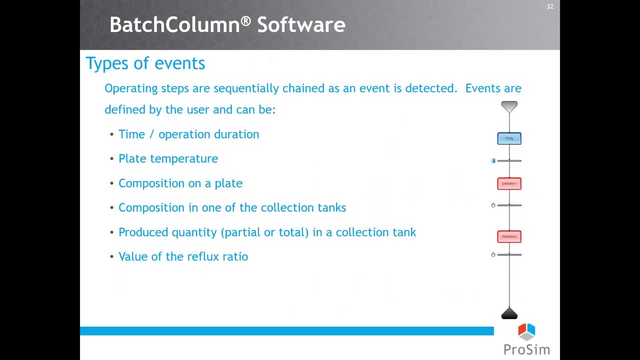 and one with variable reflux ratio. For variable reflux ratio, the software computes the reflux policy in order to maintain a component purity in the distillate. As I said before, the events trigger the end of the step, Either to stop the simulation or to move to the next step. 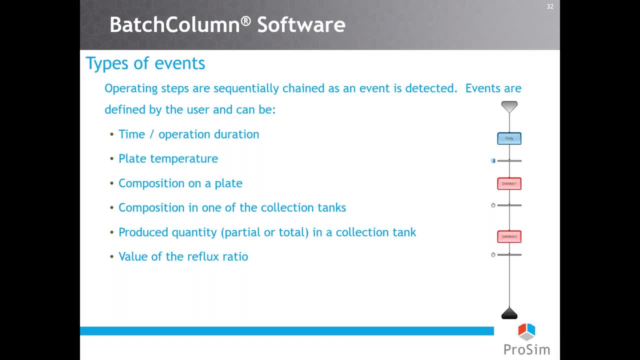 Operating steps are sequentially chained as an event is detected. Events are defined by the user and can be a simple event, like, for example, time or operation duration, but also more advanced events like, for example, the plate temperature, the composition of the plate or the composition in one. 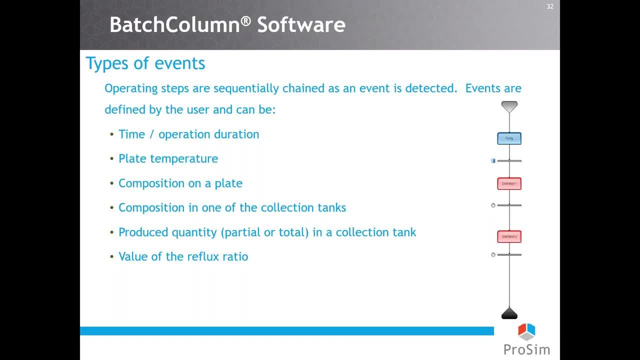 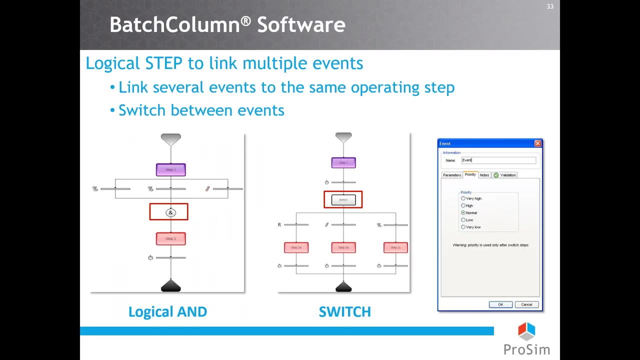 of the collection tank, the quantity which is produced in the collection tank, which can be partial quantity or total quantity- or the value of the reflux ratio. To allow you to create more sophisticated production recipes, logical steps are also available for you to introduce into the scenario. 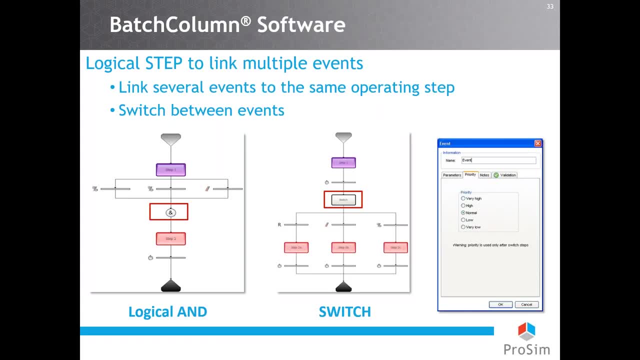 These logical steps allow you to link together multiple events which are associated to a particular step. The logical hand is used when the criteria of multiple events must each be satisfied before moving to the next step. This logical hand can only be used to link events that come from the same step, of course. 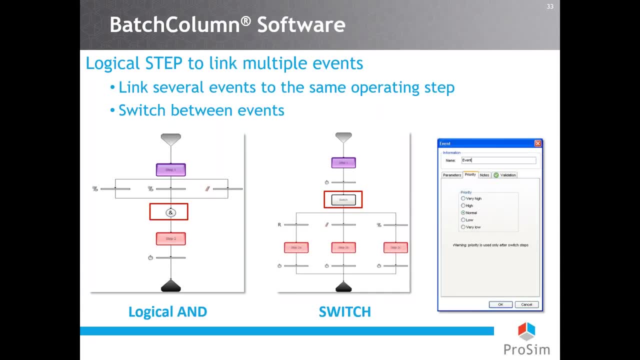 The switch element is a kind of like a fork in the road, where the next operating steps depend on which event is reached first. If multiple events are reached simultaneously, the event with the highest priority, which we define in the event window on the priority tab, takes the precedence. 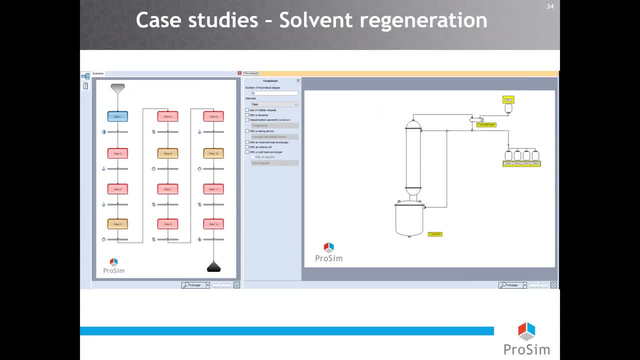 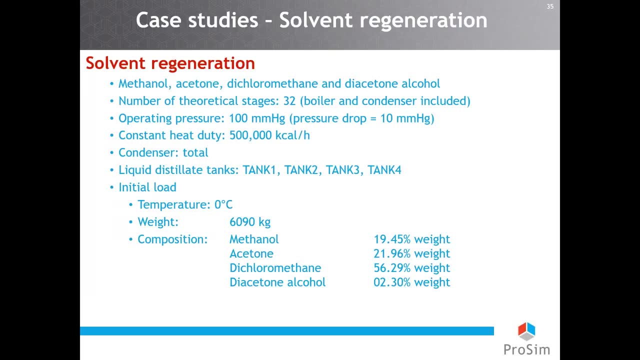 So now let's take a look at some case studies. The first case study deals with solvent regeneration. The mixture is composed of methanol, acetone, dichloromethane and diacetone alcohol. There are 32 theoretical stages, which includes the boiler. 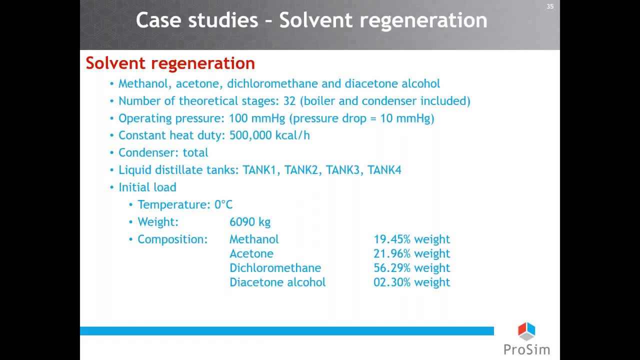 and the condenser. The batch distillation is performed under vacuum with the total condenser and the constant in duty. We have declared four liquid distillate tanks which are used to recover DCM, acetone, methanol and an intermediate cut. 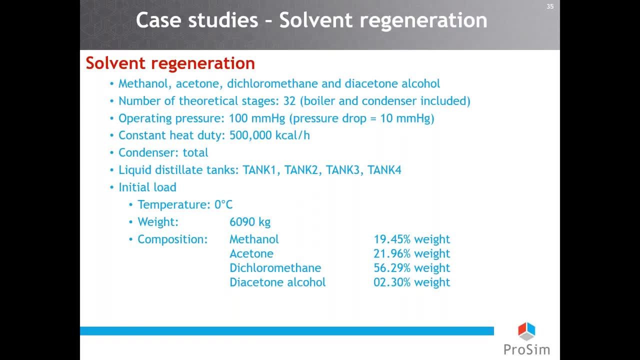 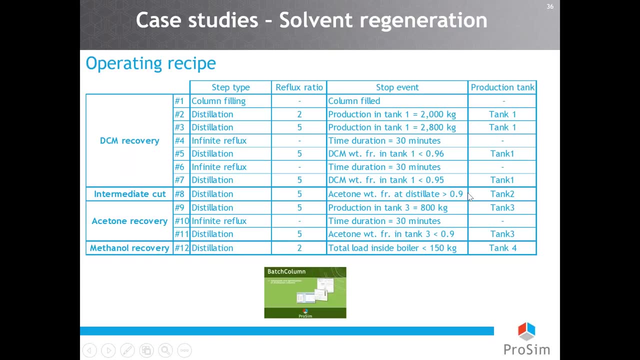 The initial load is about 6 tons of the mixture, with the composition shown on this slide. Regarding the operating recipe, it is composed of 12 steps. The first 7 steps are for the DCM recovery. First the column is filled, then there is a distillation step. 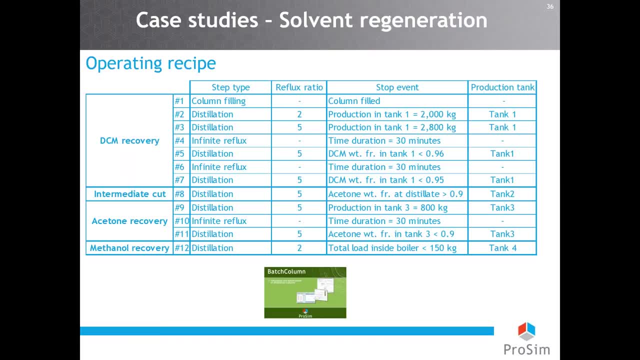 until the production in tank 1 is equal to 2 tons. Then another distillation step is done with a reflux ratio which is increased to 5 until the production in tank 1 is equal to 2800 kg. Then an infinite reflux step. 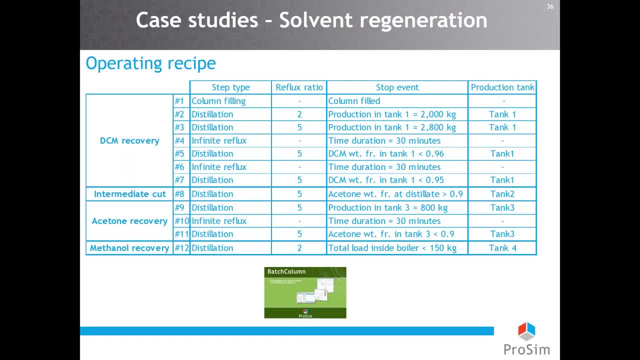 is then performed during 30 minutes, followed by a distillation step with a reflux ratio equal to 5.. The stop event is the mass fraction of DCM in tank 1.. Another infinite reflux step is done for 30 minutes, followed by a last distillation step. 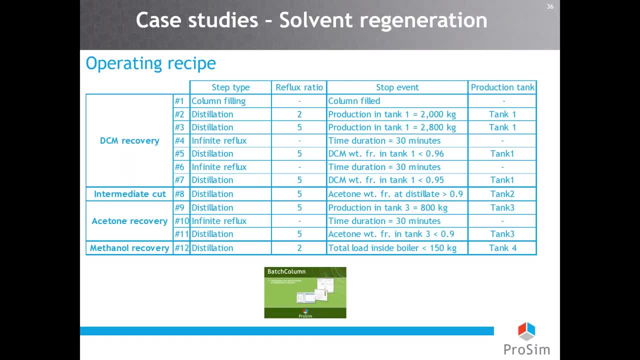 with a reflux ratio equal to 5.. The stop event is the mass fraction of DCM in tank 1, followed by a last distillation step with a reflux ratio equal to 5.. Then an intermediate cut is done using a distillation step with a reflux ratio equal to 5.. 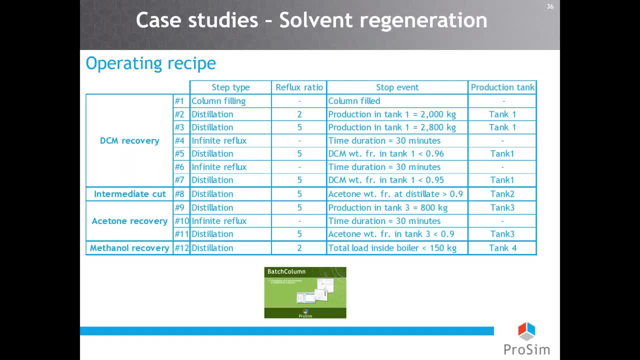 The stop event is the acetone treated in the distillate and this intermediate cut is sent to tank 2.. The next 3 steps are for the acetone recovery. A distillation step is done with a reflux ratio equal to 5.. 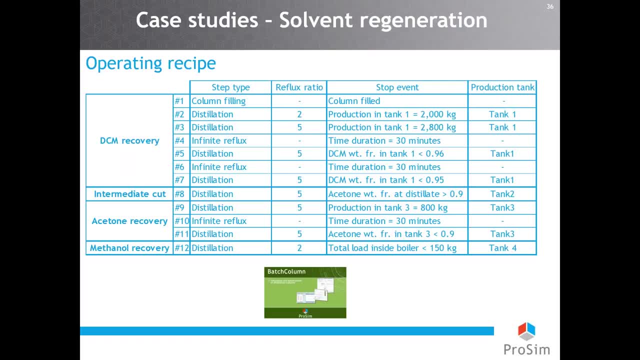 The distillate is sent to tank 3 and an infinite reflux step is then performed for 30 minutes, followed by a distillation step with a reflux ratio equal to 5.. The stop event is the mass fraction of acetone in the tank to meet the purity specification. 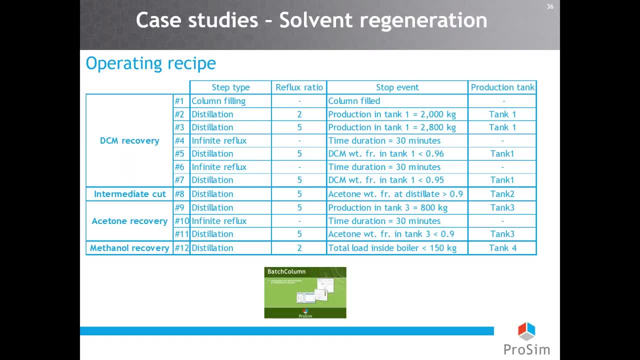 of the product. The last step of the recipe is the distillation step, with a reflux ratio equal to 2, where the distillate is sent to tank 4 and the stop event is the residual load in the boiler. Let's go through the software. 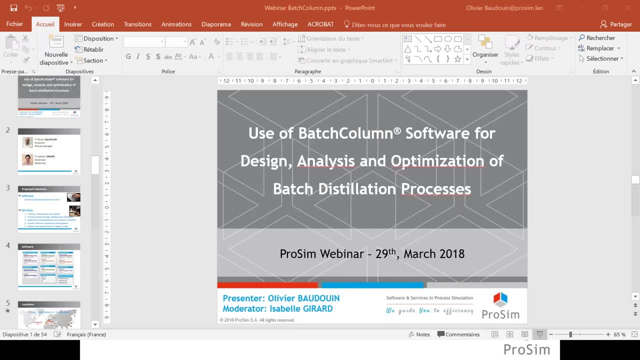 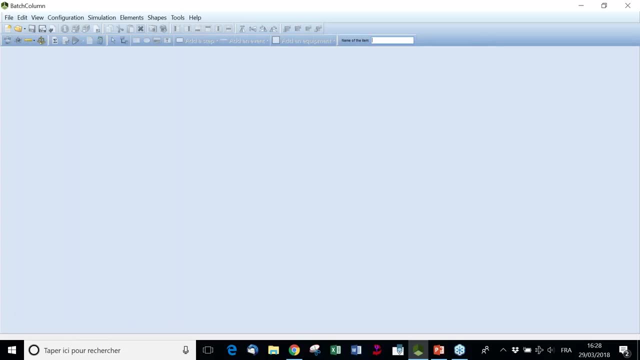 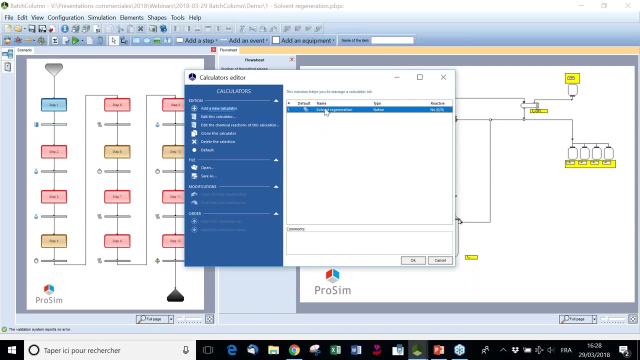 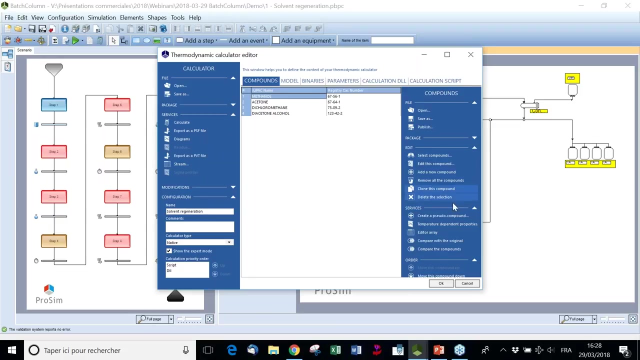 to run this case study. Here you have the thermodynamic description. This is Simulist Thermodynamics, as said before. Here you have several possibilities in order to select the component: the databases you have on the computer, for example. i've got all these databases, i can search. 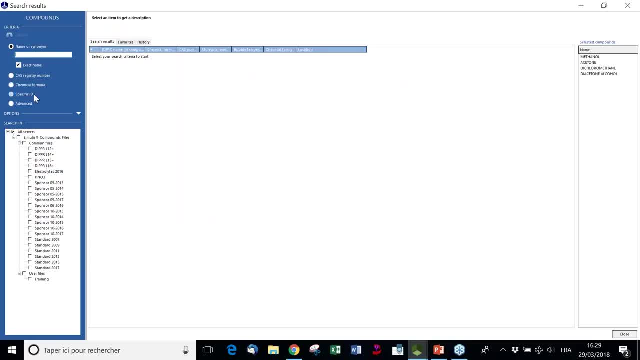 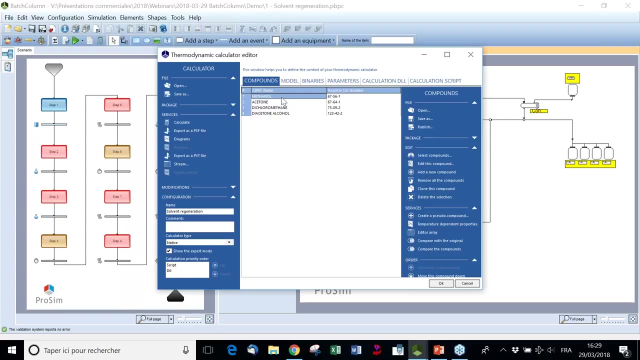 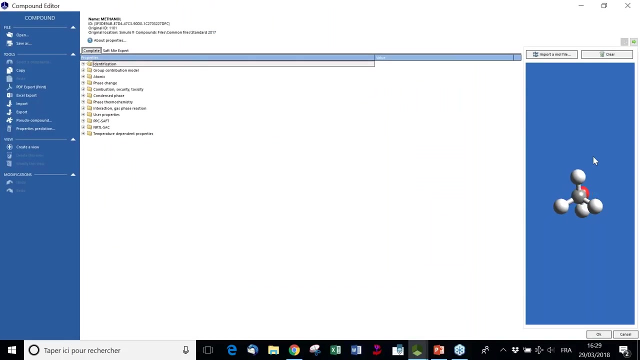 by the name, by the cast number, by chemical formula or some specific or advanced characteristics. you can also create your own components and when you have selected the the components, then you can have a look on the properties which are in the database: of course, the chemical structure, but also some information about identification. 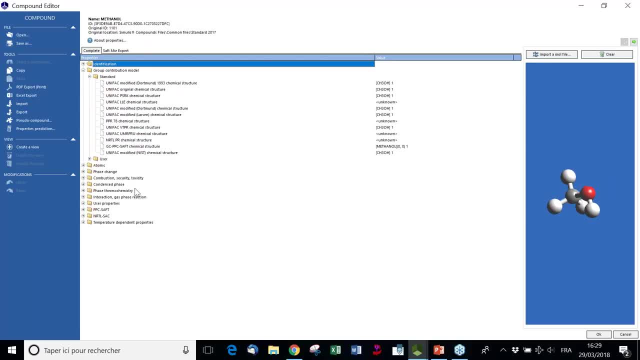 about group contribution methods. here you can see all the group contribution method we use and the corresponding group decomposition, some information about atomic properties or some properties, also about phase change, for example critical temperature or critical pressure. what you can see is that, using the software component approach, we include software. 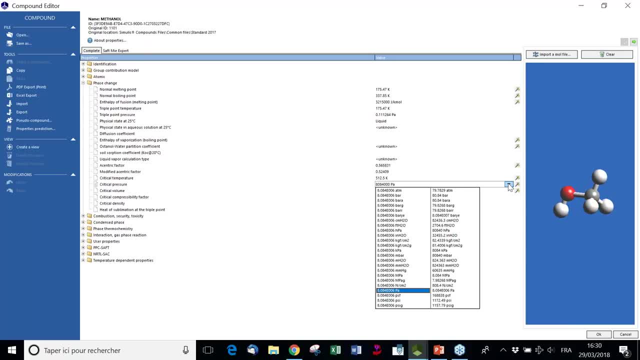 for the unit conversion. and here, for example, if you have the this value in terms of pascal directly, you have all the conversion in the other units which are available in the system where you see the magic ones. that means that we can estimate the properties, pure component properties, from the chemical structures. 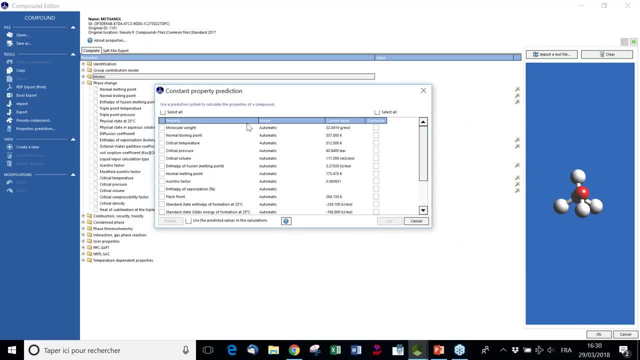 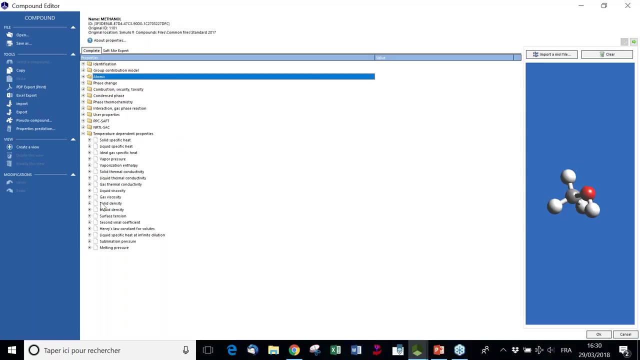 and to do that, in fact, here you have several methods and you can select from different predictive methods which one you want to use to predict your pure components, if the components you want to use is not available here, available in the databases. We also have some temperature-dependent properties. 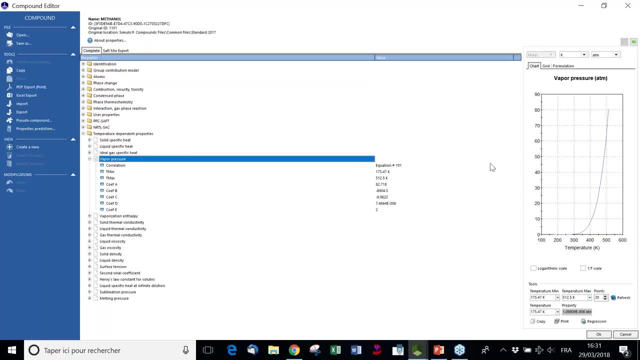 For example, let's have a look on the vapor pressure, which is very important for distillation, And here what you see is the equation we are using. If we go on the right of the screen, you see the corresponding equation with the temperature. 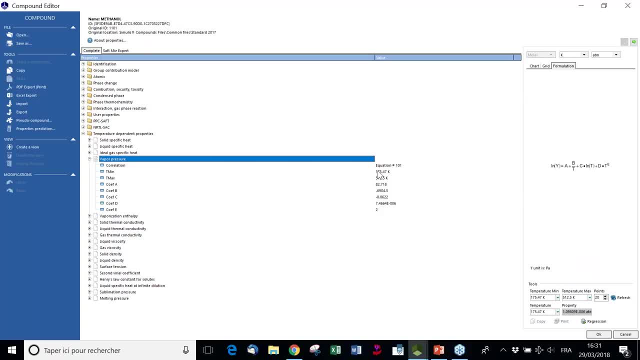 range, validity and the corresponding parameters A, B, C, D and E. in that case, Here you have a chart and the grid of the calculated values, And for the chart you can change the scale if you need And of course, you can change also the units. 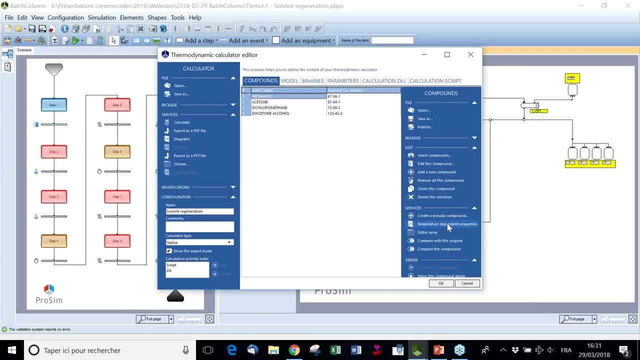 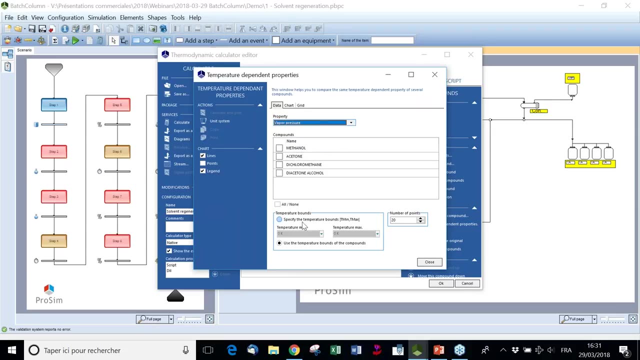 You can also do some. We have some services, For example to compare the components we have inside the calculator. For example, we can compute all the temperature-dependent properties using the vapor pressure And we select all the components in that case And then one can see which are the more volatile components. 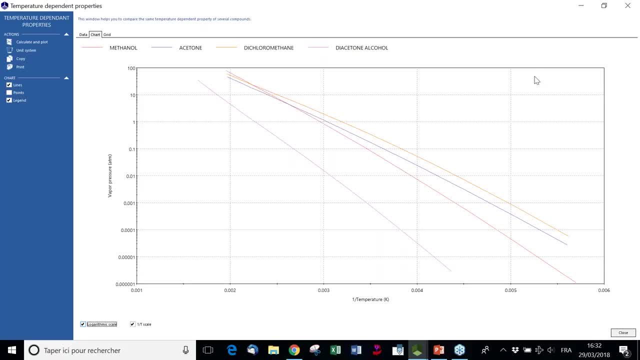 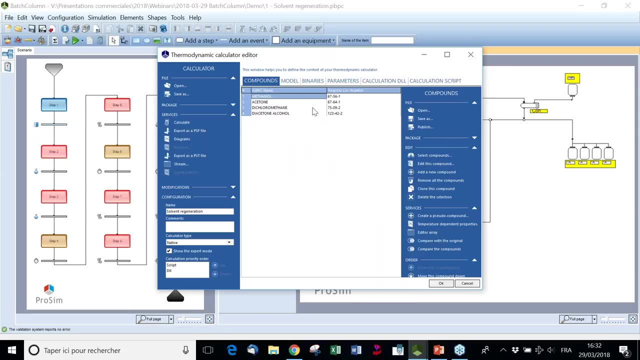 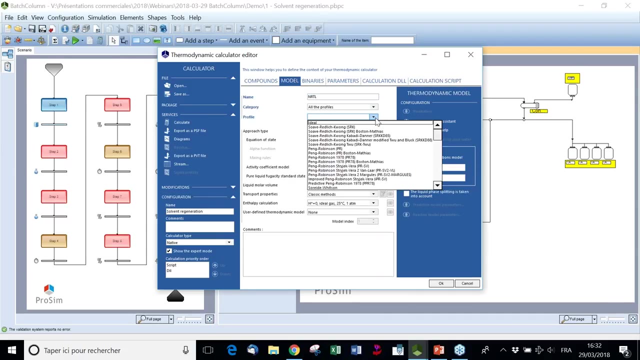 We can see if we have some bone growth points, for example, and so on. Okay, When you have selected all the components which are in the mixture, then you have to select the model that you want to use with. Here you have different predefined models. 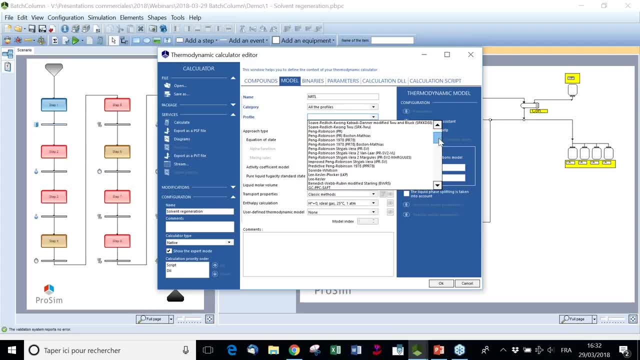 As I said before, which can be equation of state activity coefficient model, combined approach of specific models. You can add also several categories for these models. Okay, And here we have the whole equation. Okay, If you are using, like in that case, an RTL model, you need some binaries. 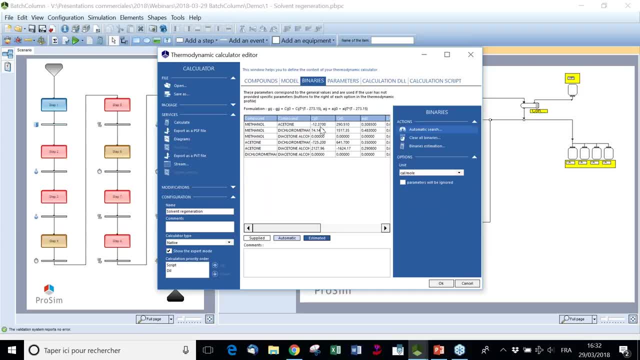 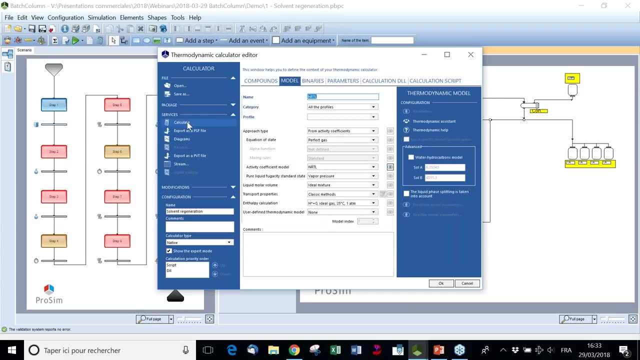 The binaries can be searched from databases provided by the user or estimated using one of the predictive models we have, for example UNIFAC models or COSMO models. Then, when you have selected the components, the model, then you can use some calculation services. 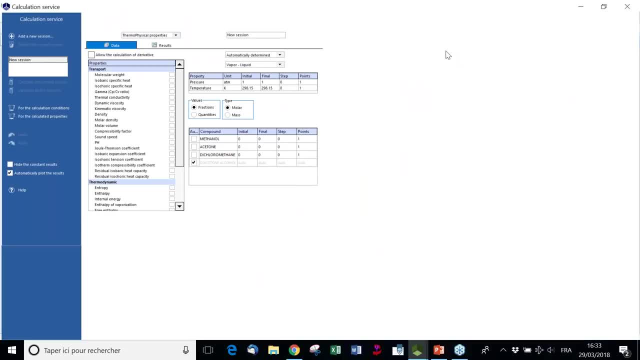 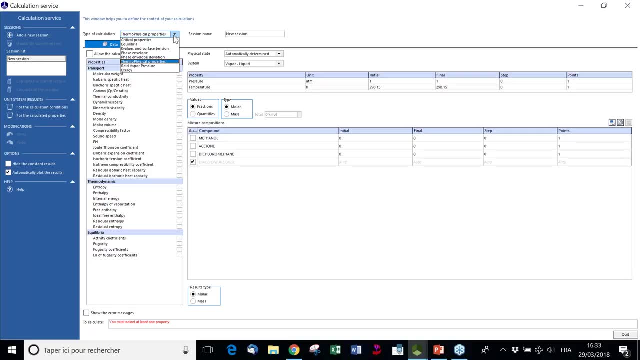 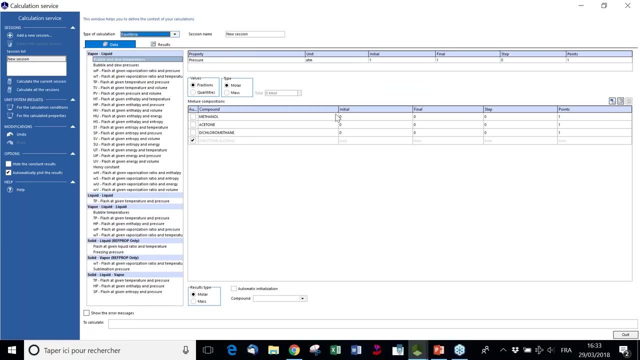 like, for example, the service calculation and you can compute thermophysical properties or, for example, equilibria calculation. In that case, for example, we will do the calculation of the bubble and dew temperature at atmospheric pressure for the mixture methanol with DCM. 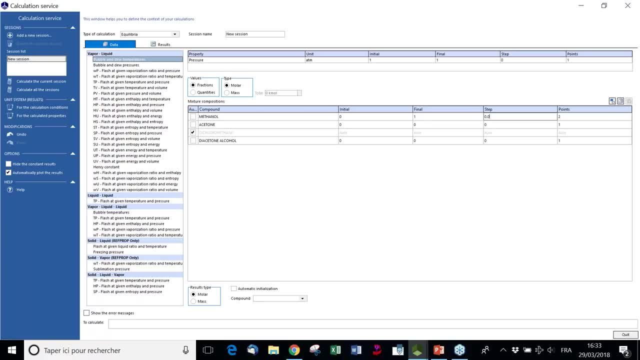 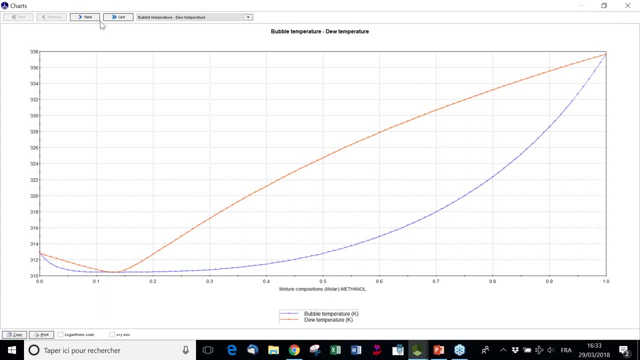 I will vary the composition of methanol from zero to one. that means 100 opoints. Then I run the calculation, and here I can see that I've got an azeotrope for this mixture. So here you have the bubble temperature. 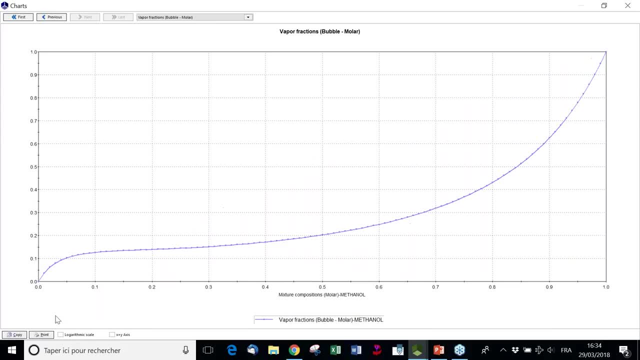 Here you have the dew temperature. You can go to the variable fraction with respect to the liquid molar fraction. and here you can see the dew temperature. Here you can go to the variable fraction with respect to the liquid molar fraction. Here you can go to the variable fraction with respect to the liquid molar fraction. 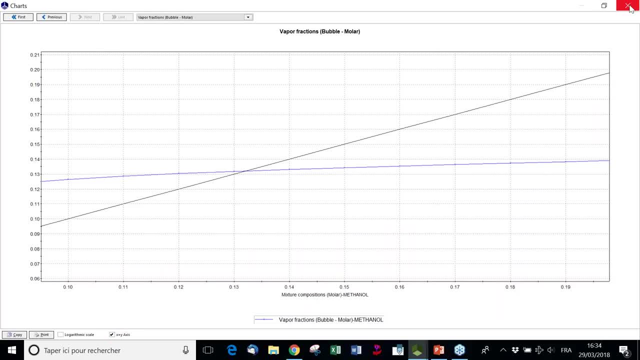 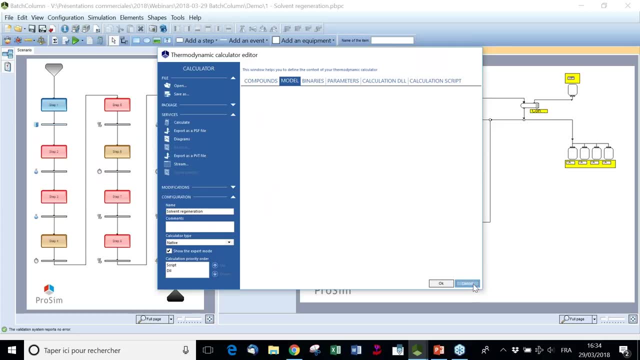 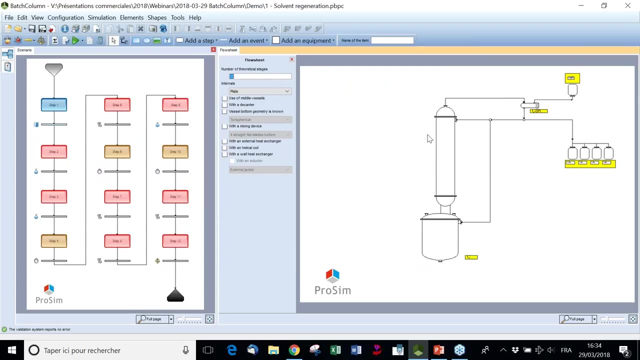 Here you can go to the variable fraction with respect to the liquid molar fraction. So when the description of the thermodynamics is okay, then you can go to the description of the process. So in that case, as I said before, we have a column which is very simply described. 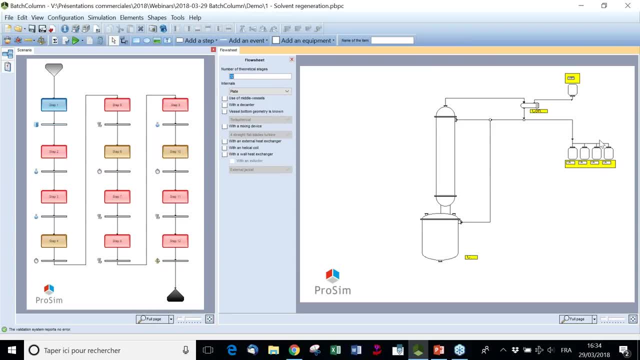 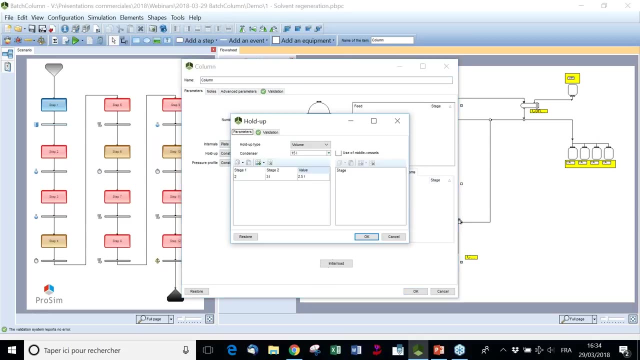 This is the first case. We describe four production tanks. We put a number- All that is assumed to be known- for the condenser and also for all the stages. Same for the pressure profile: We provide the top pressure at the condenser and the remaining pressure drop. 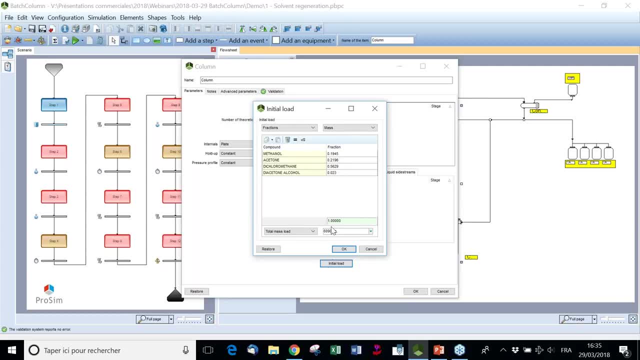 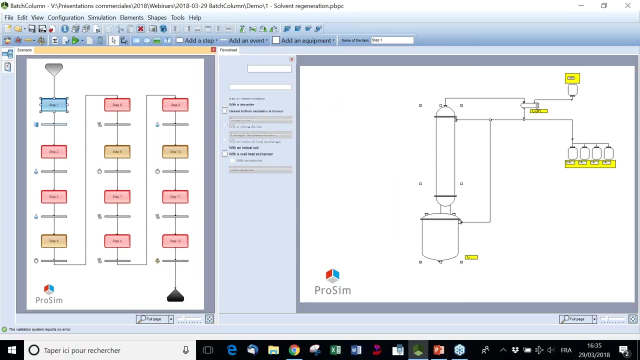 Here we describe the initial load, That means the total mass load and also the fraction. Of course, you can select what you want. it could be a mole fraction, volume fraction and so on. Then you describe the operating recipe, or what we call the scenario. 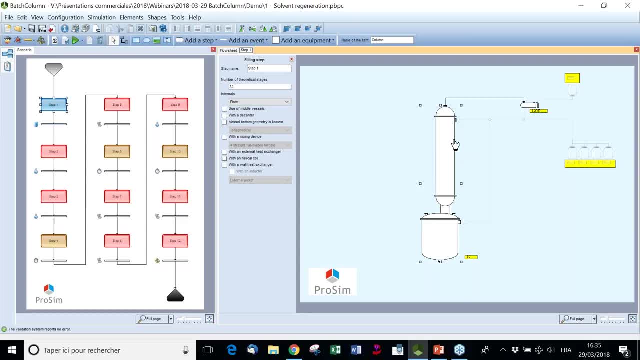 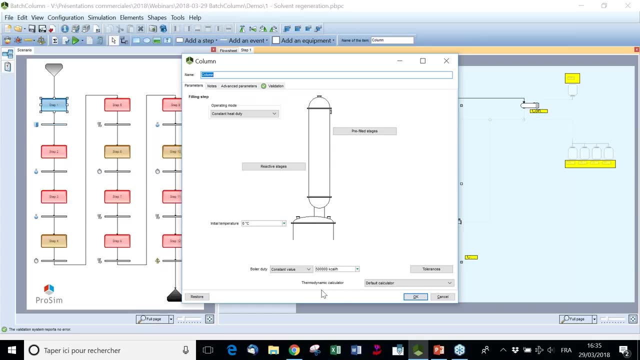 For the first step. this is a step which will fill the column, So in that case we only have to provide what is the heat duty that we provide to the condenser, To the boiler. We could provide some pre-filled stages in that case. this is not the case. 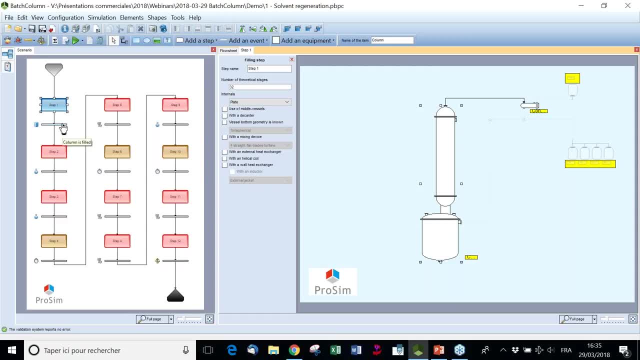 For that step the stop event is automatic. That means that we will detect when all the stages are filled. Then for the second step, as you can see, we select the tank 1 for the production and we provide the reflux ratio and the heat duty. 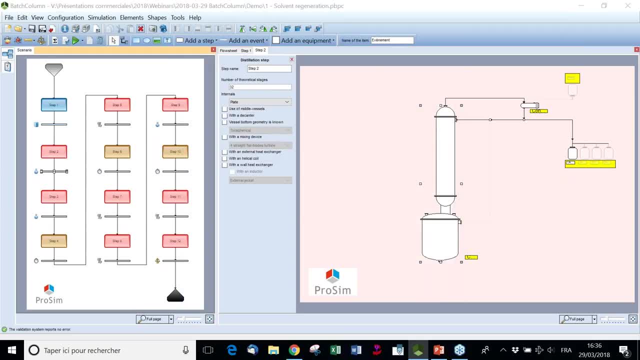 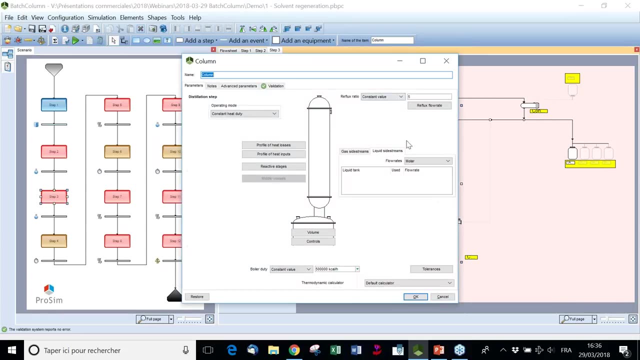 And for the event, we select the total production inside the tank, which is the tank 1, and which should be equal to 2,000 kilograms. We do the same for the step 3.. Here, as said before, we increase the reflux ratio. 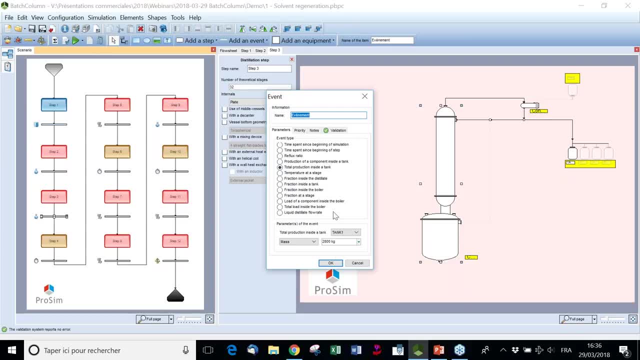 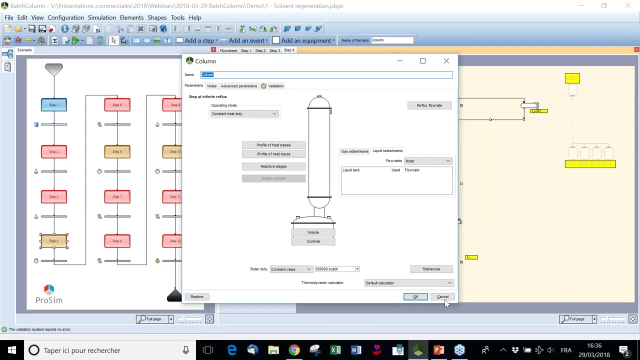 The stop event is still the total production inside the tank, which is 2,800 kilograms. Then we add the reflux ratio, Then we have an infinite reflux step. In that case the reflux is infinite and we only have to provide the heat duty at the 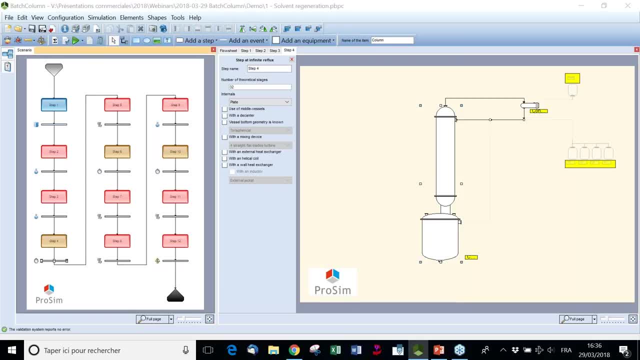 boiler. The stop event is the time spent since the beginning of the step- 30 minutes. Then the step 5, we come back with a reflux ratio of 5.. Still, the production tank is the production tank. Then we add the reflux ratio. 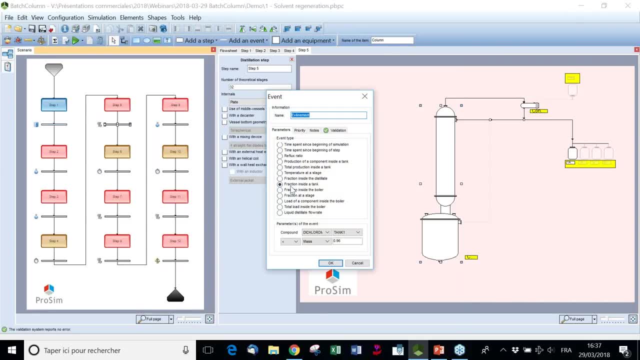 There you have the Tom Key, the standard reflux ratio. Then we have the reflux ratio, We do the same, and now we have to add the reflux ratio Instead of the stink factor, which is the 1. And we will solve the formula. and now we apply this sitting in order. 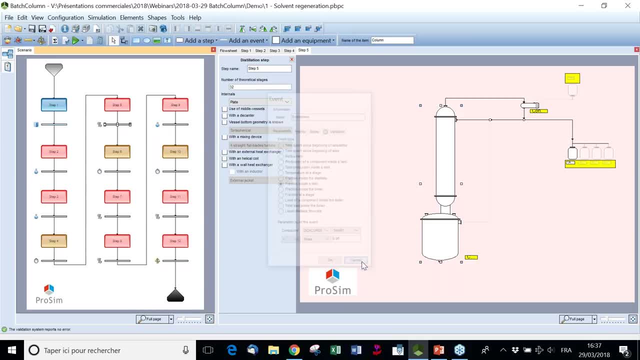 It is the same. We double the refeminize, which is equal to 6. Then we add the reflux ratio, We complete the피iez diferença. Then, in any case, we will have a Uง demand change for the next while meeting. 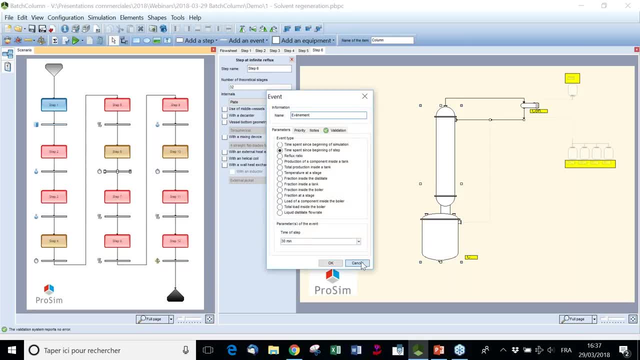 Then we have to calculate the reflux ratio for this tank 1.. So we will take the reflux ratio, we convert it to the tanks, We put the reflux ratio above the tank 1.. And the last, for this time we are going to figure out whether we want an infinite reflux. 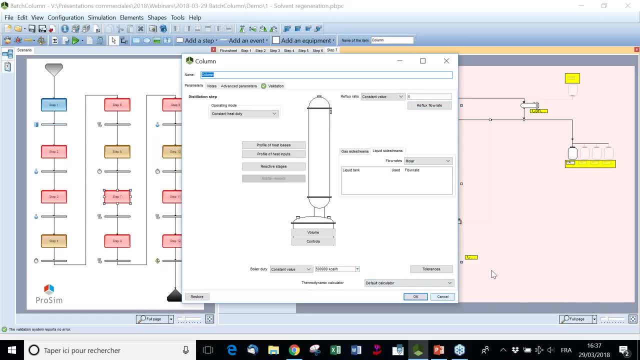 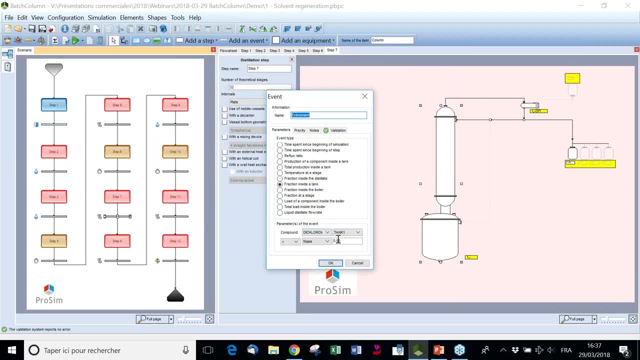 ratio for another oil tank or not. we have reflux ratio equal to five, still a production in tank one, and we stop when we reach the fraction inside the tank one. Then, for the steps eight, we switch to the tank two. Same parameters are equal to reflux ratio equal to five. 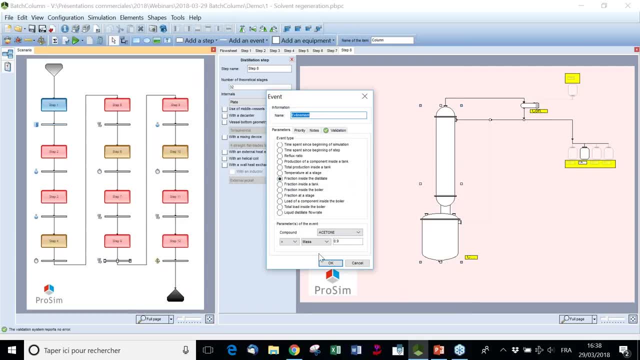 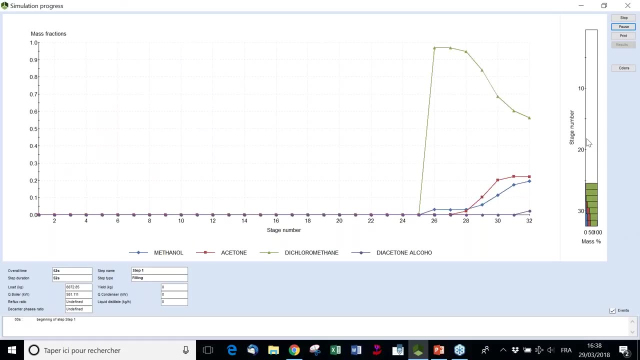 Then the stop criterion is the mass fraction inside the tank. two and so on. So when you describe all the recipe then you can run the simulation. So on the right side of the screen here you have the composition of the boiler And what you can see is how the components are growing from the boiler to the top of 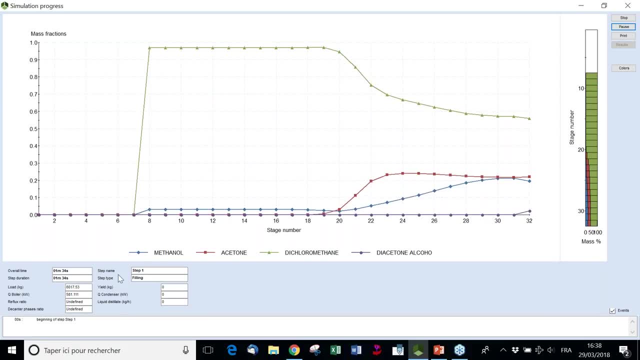 the column And you can see that you have all the stages which are filled, one after one. So here you have the name of the step, Here you have the step type. So now we are in the step two, which is distillation. 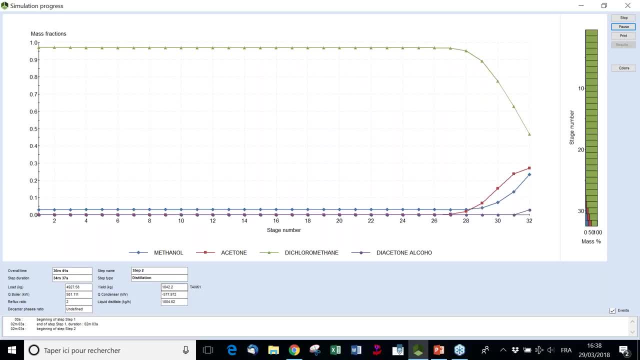 The pollution is tank one. Here you have the load, Here you have the time, Here you have the step duration. So we switch to step three. The reflux ratio is equal to five. Then step four with total reflux. you can go that. you can see that components are going. 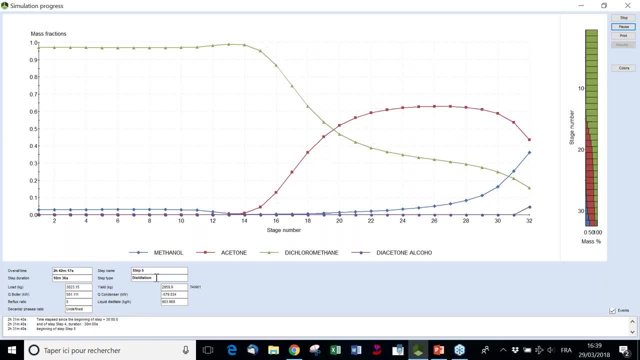 to the boiler: Step five, Step six, infinite reflux. Step seven: still distillation in tank one. Then we switch to tank two, tank three, infinite reflux, Still a distillation step, Step seven, And then we reach the final event, which is the load in the boiler. 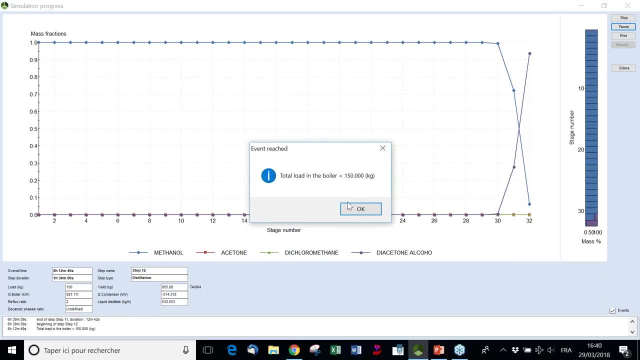 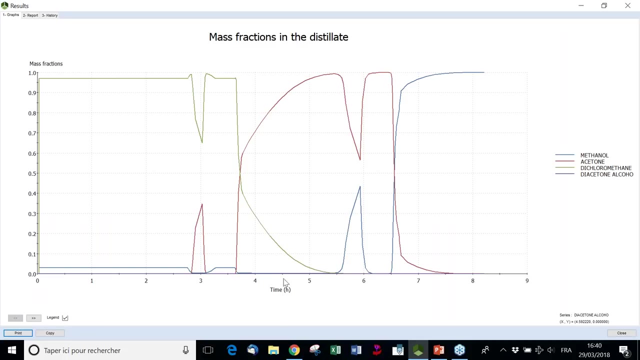 And then we reach the final event, which is the load in the boiler. So here we have the results with respect to time. We have the mass fraction in the distillate with respect to the time for the dichloromethane for this time. 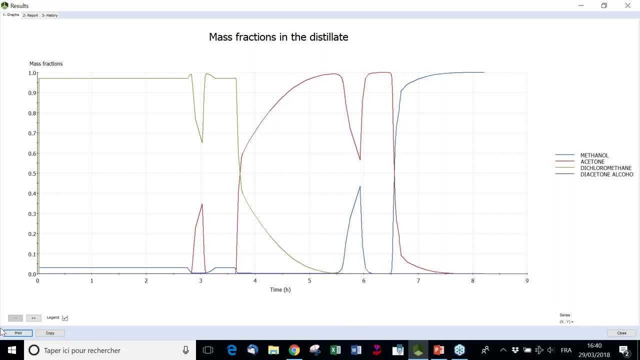 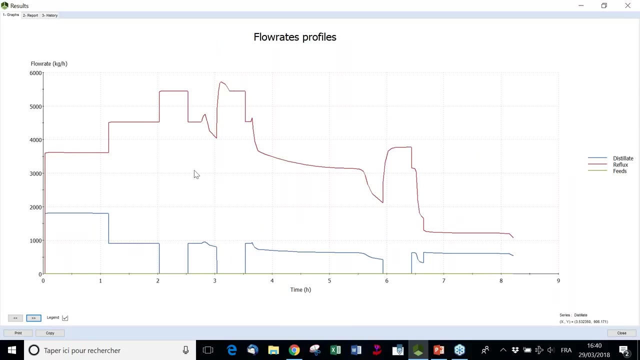 And then we have the reflux ratio, We have the acetone in red, and so on, Same. we have the mass fractions, evolution with respect to time in the boiler. Then we have information about the fluoride profiles for the distillate, for the reflux. 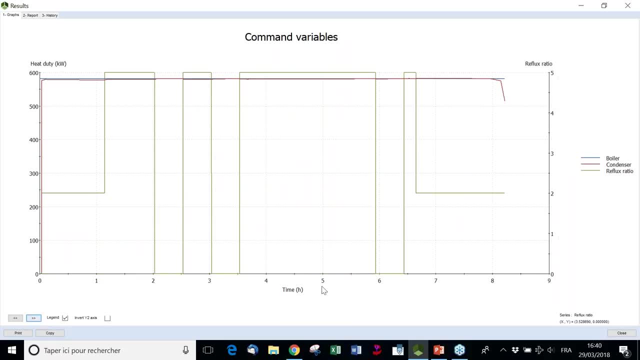 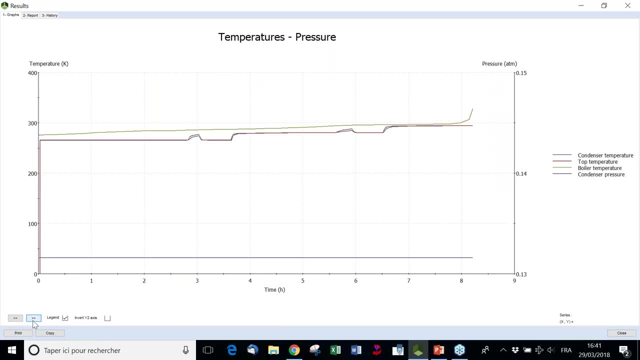 And in that case we don't have any feeds. We have also information about the reflux ratio and heat duty for the condenser and for the boiler. Here you have the reflux ratio. Here you have information about the temperature, evolution of temperature in the boiler or 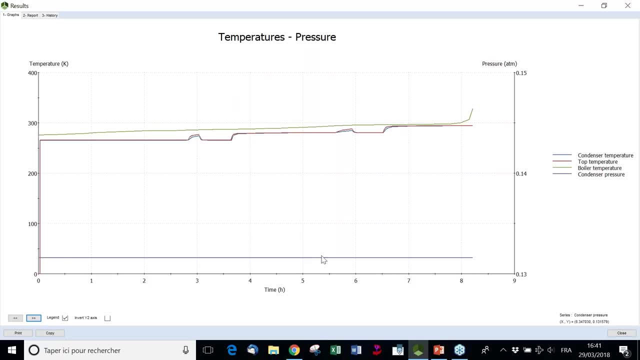 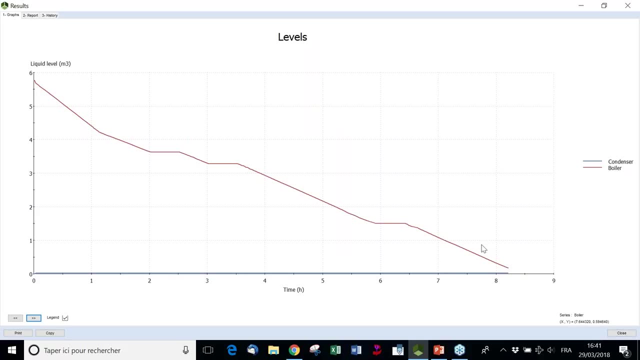 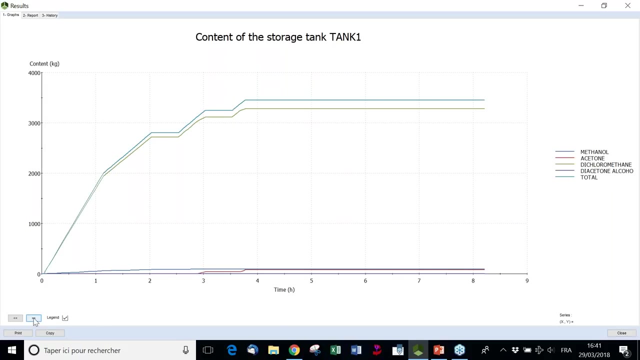 at the top and in the distillate. The pressure in that case is constant. Then you have also information on the level in the boiler and in the condenser And you have information about all the storage tank. For all storage tanks you will have information about the content. 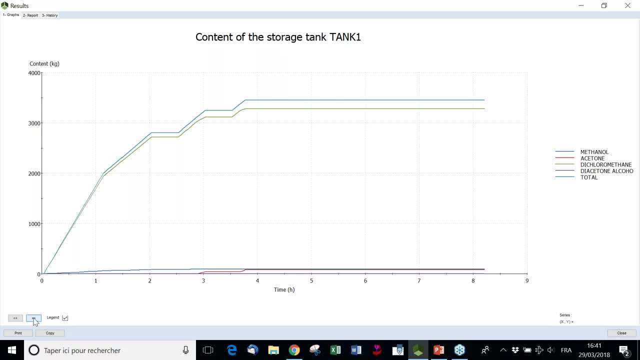 That means kilogram of compounds, And then you have the reflux ratio, And then you have the reflux ratio, And then you have the reflux ratio And also in terms of mass fractions. So this is for tank one, Then for tank two, which start the feeding at after three and a half hour. 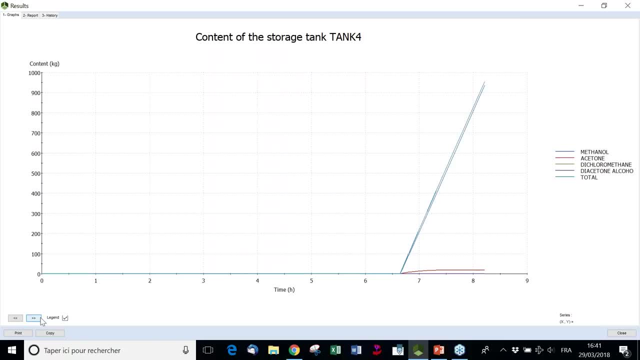 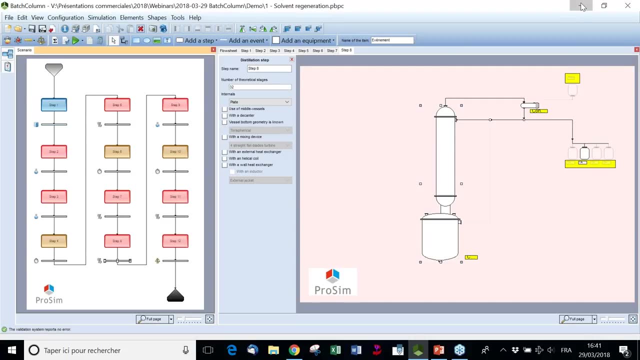 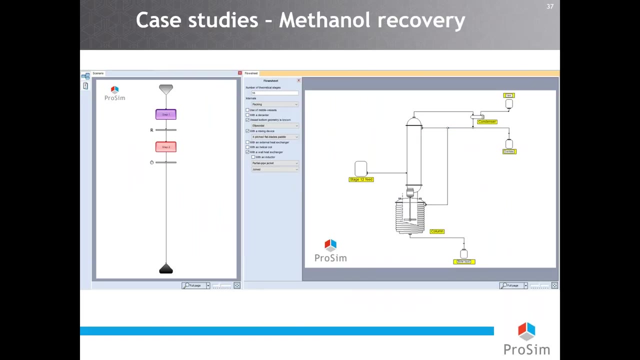 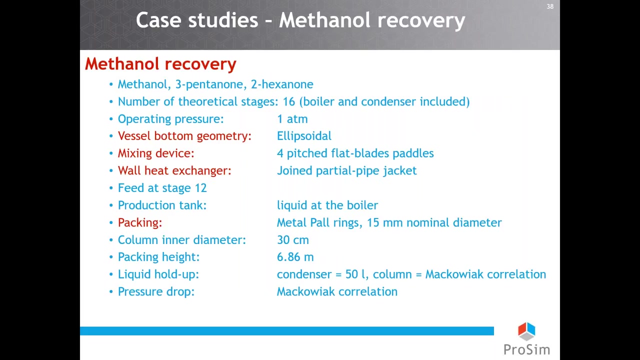 Tank three And tank four. So this is a very simple example. So come back to the presentation. So the next thing, So the next thing, So the next example is the methanol recovery, And this is from a mixture of methanol, 3-pentanone and 2-hexanone. 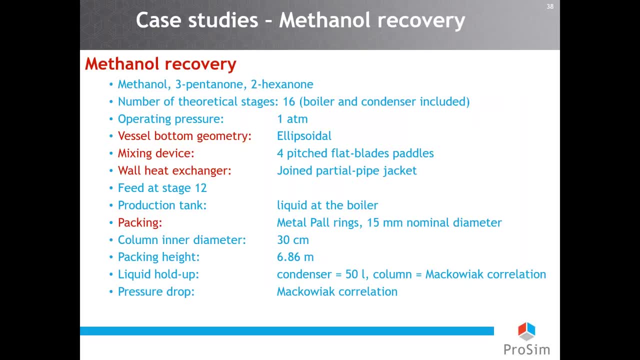 We have 16 stages, including the boiler and the condenser, And in this case the vessel geometry, the mixing device, the heat exchanger and the packings are described in details. Thus, the heat flux, the liquid holdup and the pressure drop are computed from this characteristic. 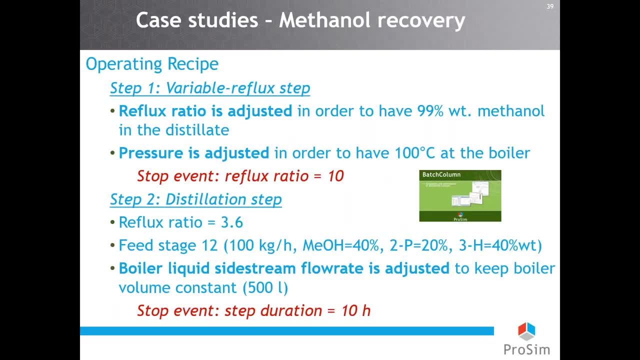 So these are the resources, these characteristics. Moreover, we will have some controls. That means that the step 1 will be a variable reflux step. During this step, the reflux ratio is adjusted by the software in order to have 99 weight percent of methanol in the. 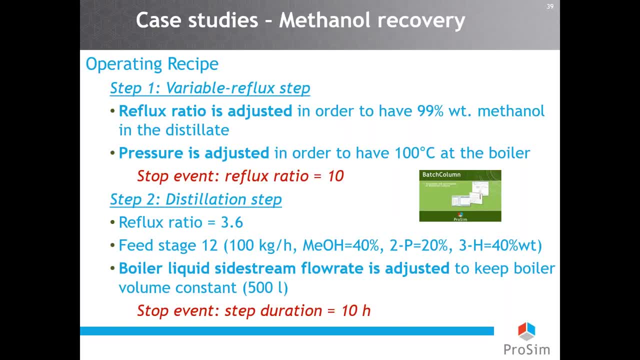 distillate. The pressure is also adjusted so that the temperature in the boiler is equal to 100 degrees Celsius, And the stop event of this step occurs when the reflux ratio is equal to 10. Then the second step is a distillation step at. 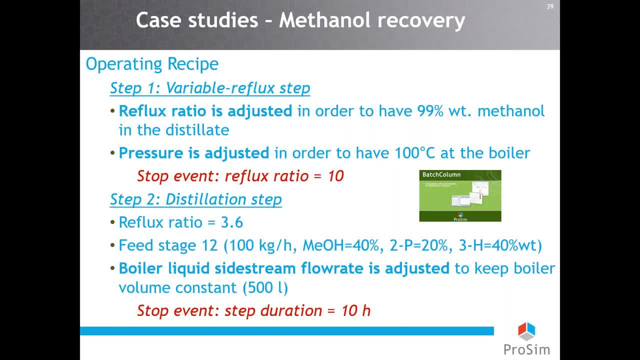 fixed reflux ratio. A feed of 100 kilogram per hour containing 40 percent of methanol, 20 percent of 2.9, and 40 percent of 3 hexanon is found on stage 12 of the column And the pressure is still adjusted in order to have 100. 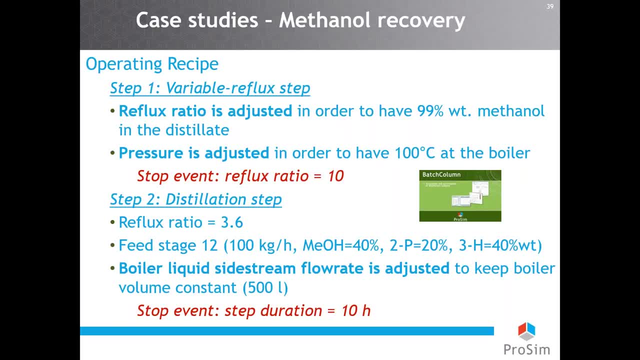 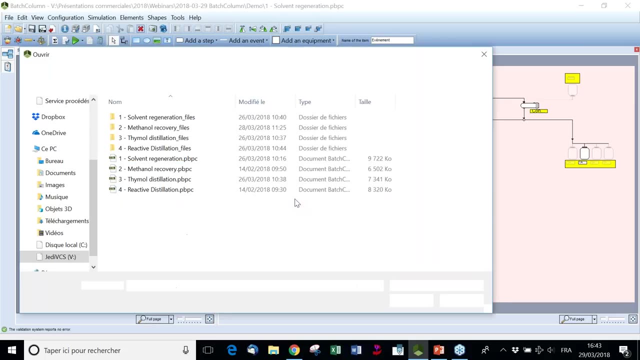 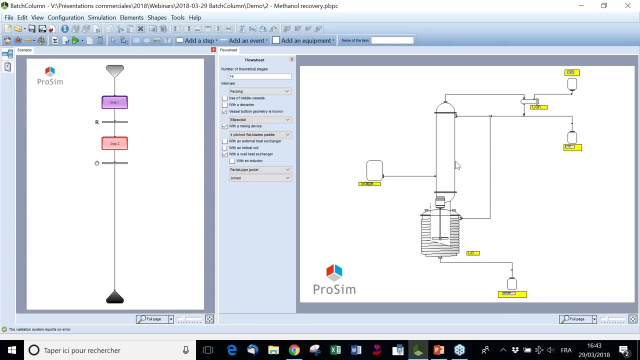 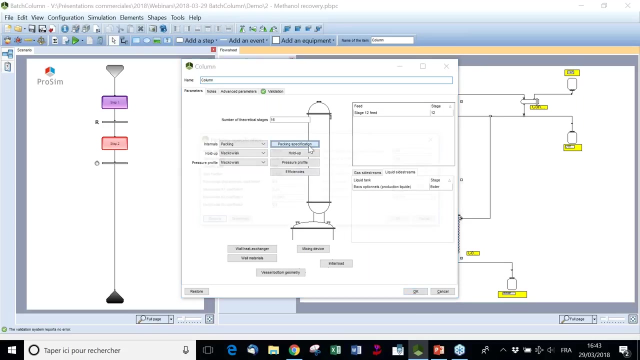 degrees Celsius at the boiler And the boiling. the boiler liquid size 248 is also varied to keep the boiler volume constant. And these steps last 10 hours. So now let's go to the software to see the demo for this corresponding example. So in that case we provide the packing specification. 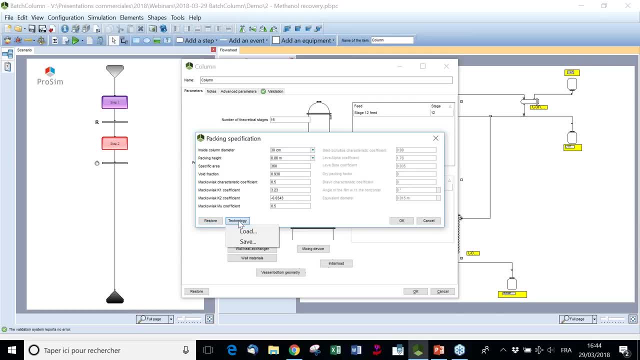 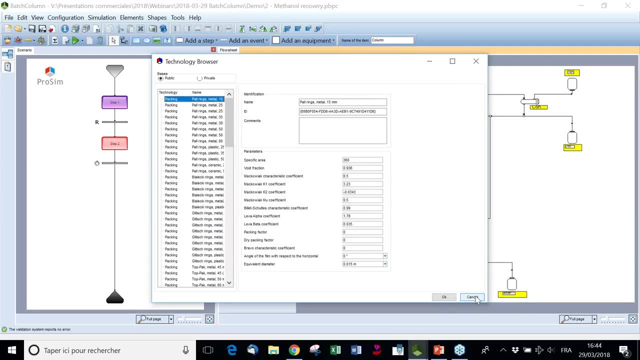 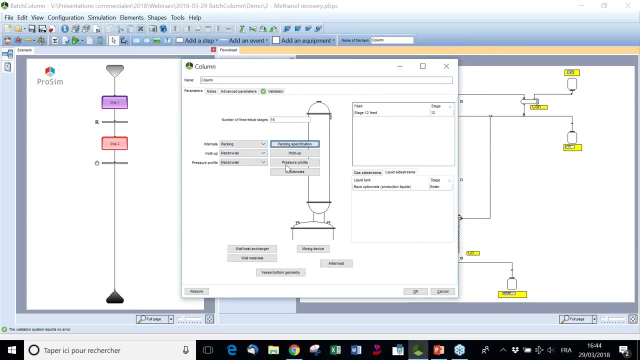 The packing specification can be loaded from the technology. as said before, Here you have a library. You can add your own package if you need. You can have a private database And we will have correlation to compute the holdup and the pressure profile. 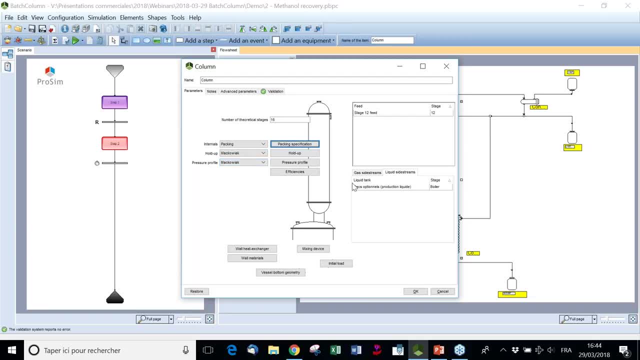 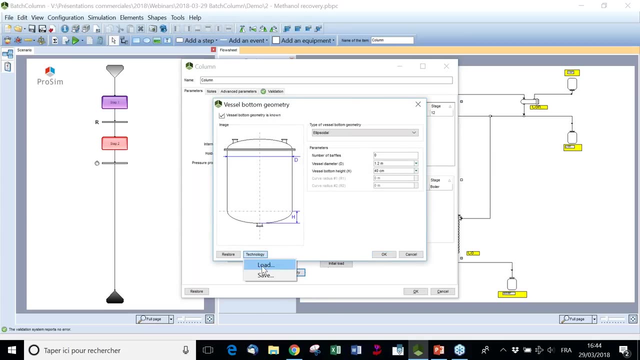 We will provide, of course, the initial load, the one I described before, Then the vessel button- geometry. Still, you have a technology button here to load from a library which vessel you want to use. You have information about warm materials. In that case, we only have one material. 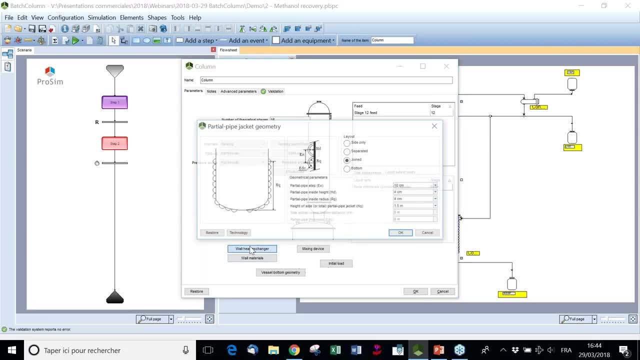 You have information about the water material, In that case we only have one material. You have information about the material, In that case we only have one material: the wall heat exchanger. in that case this is partial pipe jackets which are joint with these characteristics. here also you can load everywhere you can. 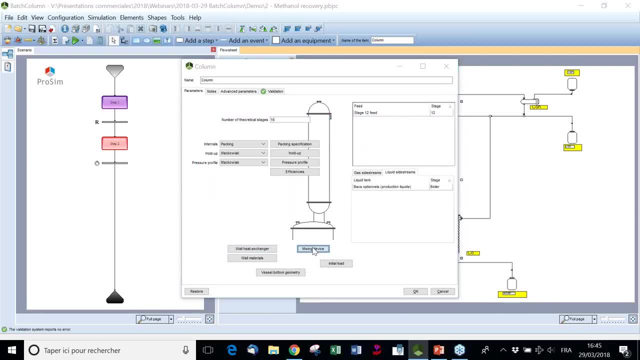 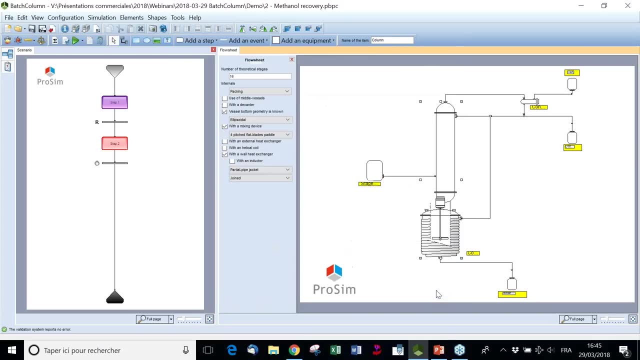 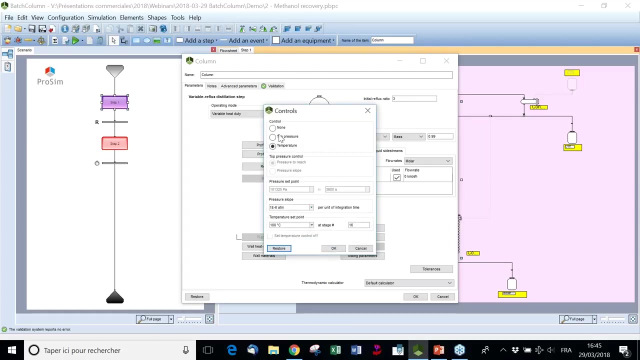 load from the technology button and the mixing device. this is a four pitch flat blade puzzle. then we have the first step. in that case the feed is not open. here we describe the controls. that means that we want the temperature to be equal to 100 degrees Celsius at stage 16. that means in the boiler. we start from a. 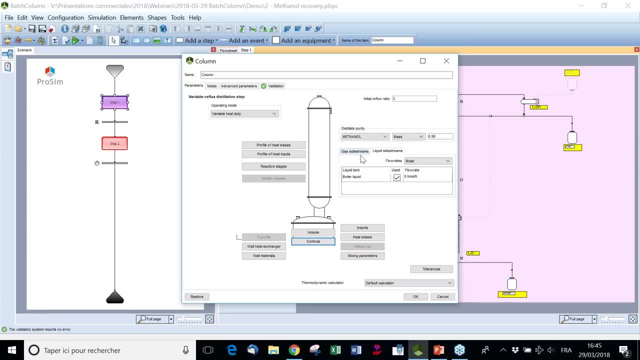 reflux ratio equal to 3 and we want to keep this distilled purity, so we will adjust- the software will adjust- the reflux ratio in order to keep this purity. for the wall heat exchanger, we have to describe which utility feed we are using. it could be water or saturated steam, or 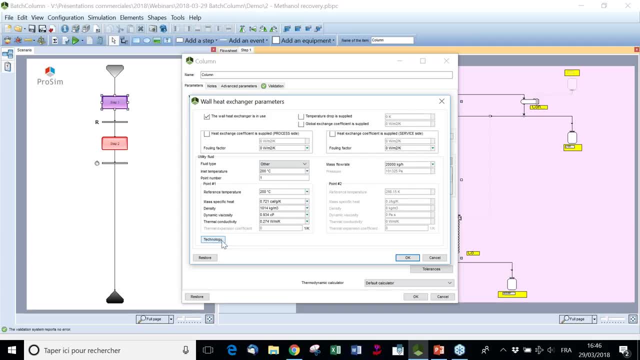 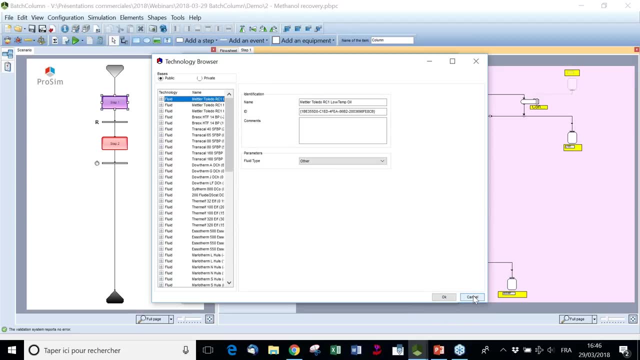 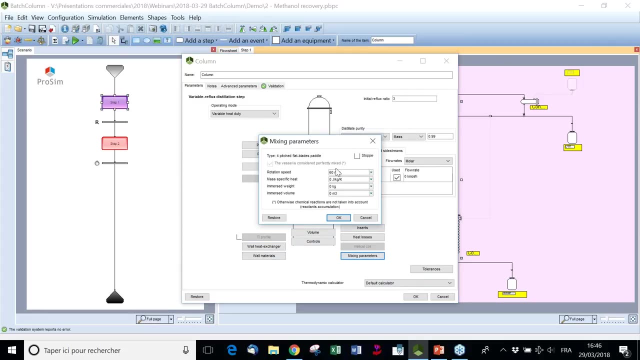 if it's, what is it other? that means that you can load from the technology here some, some specific freeze and regarding the, the mixing parameters, here you only have to provide the rotation speed which will have an impact on the heat exchange coefficient and the event we described here. we have the reflux ratio which is equal to 10. then that 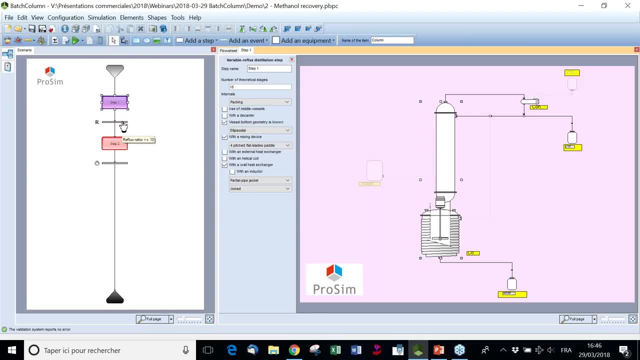 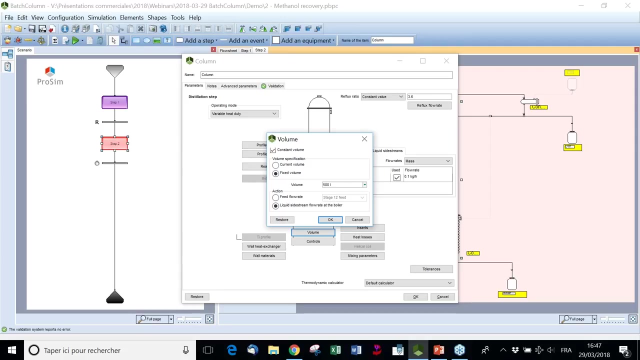 means that when this reflux ratio is reached, we will go to the next step. for the second step here, the, the, the feed is open with this composition and this flow rate. here we describe that we want a fixed volume at 500 liters, acting on the liquid size size stream. 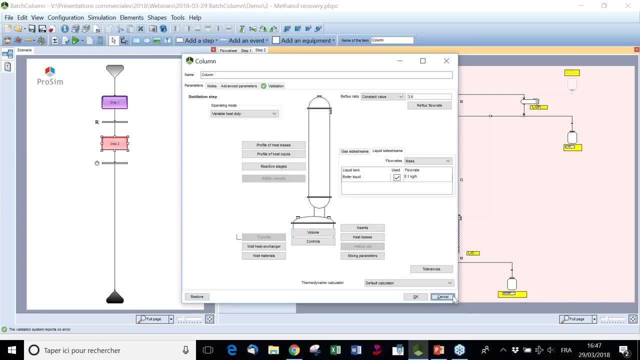 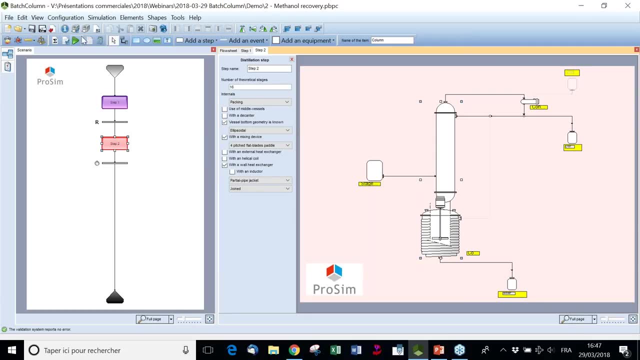 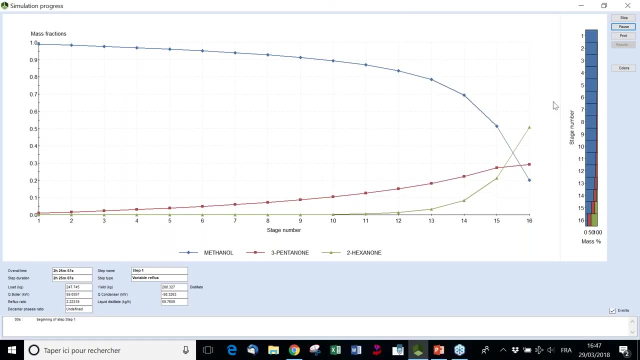 flow rate and the event is the step, which is equal to 10 hour. so now let's go to. you can run the simulation, so in that case we start from infinite reflux. okay, so we have simulated the 13 hours. then let's go to the results. here we have the mass fraction in the distillate. 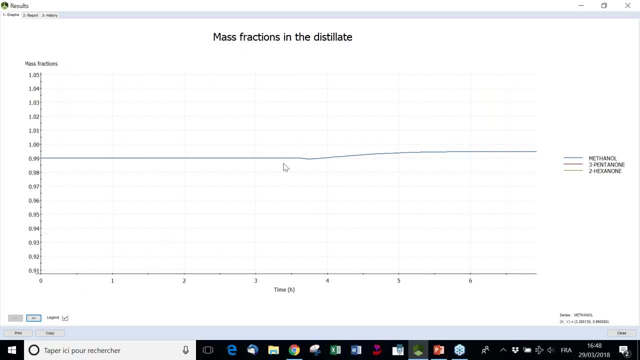 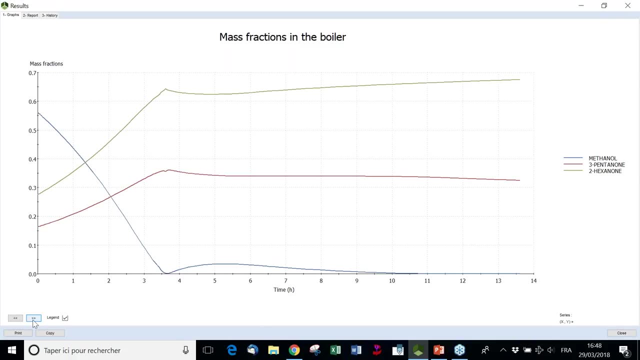 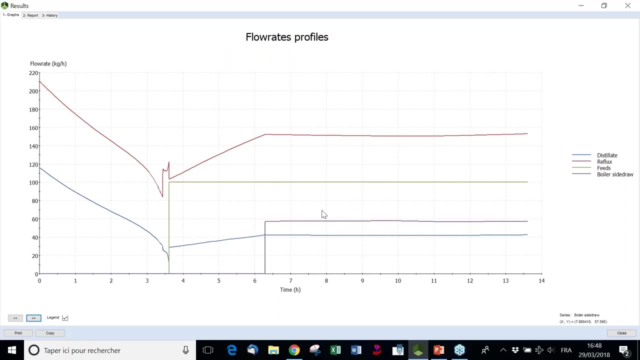 if we do zoom, we can see that this is constant during the first step. here you have the mass fraction in the boiler. here you have the flow rate profiles. you can see that we have start the boiler side stream in order to keep the, the volume of the. 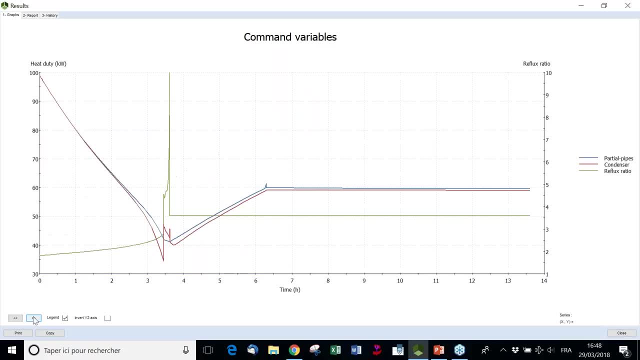 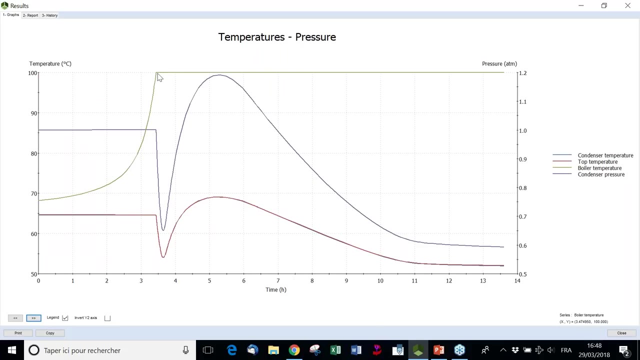 boiler constant. here, regarding the current variables, you can see that the reflux ratio is increasing to 10, and then we switch to the next step, for the temperature and pressure. the temperature is increasing to 100 degrees celsius, and then the control is done with the pressure. 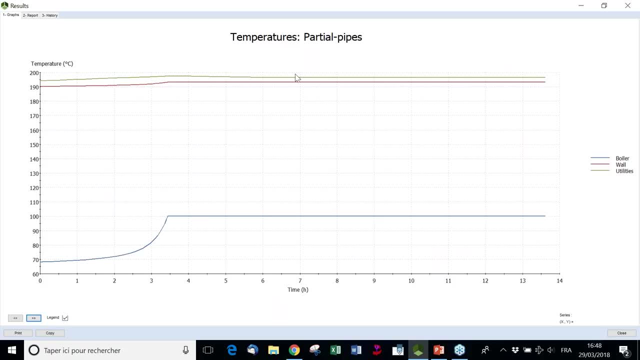 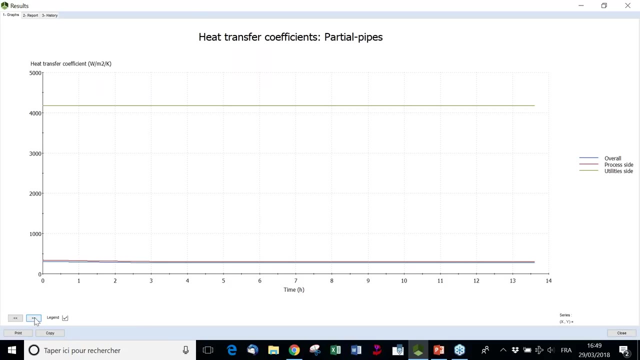 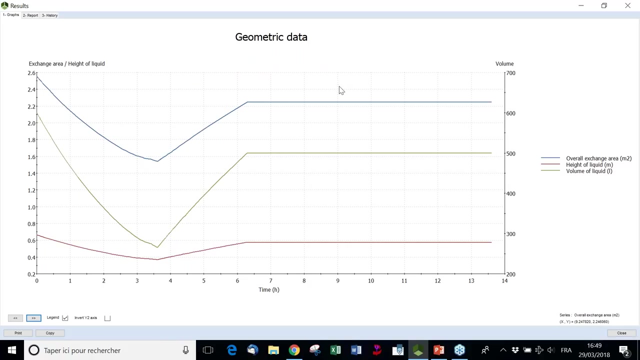 here you have information about partial pipes, about the boiler temperature, which is control, and the wall, the partial pipe, the utility. here you have information about heat transfer coefficient, which are calculated by the software. here you have information about the heat exchange area, which evolved because the the volume of the liquid in the boiler is changing. 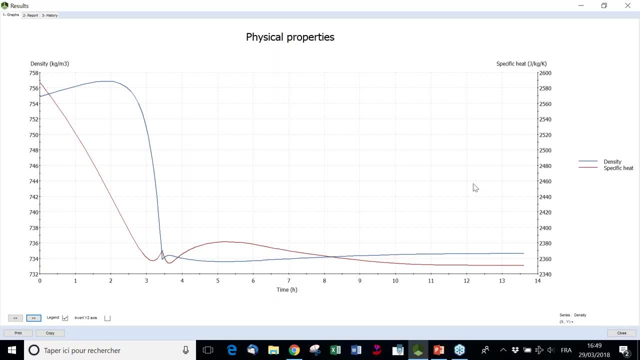 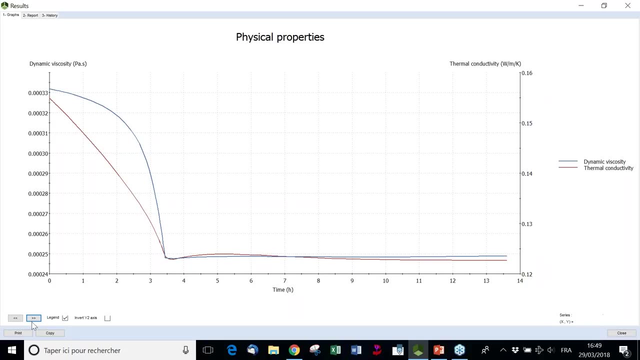 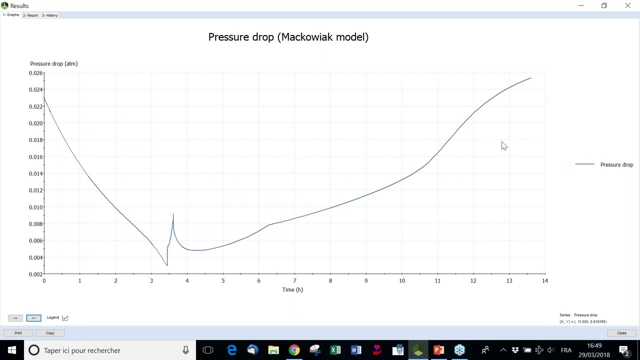 here you have the evolution of the physical properties for the, the density, the specific gravity and the dynamic viscosity and thermal conductivity. here you have information about boiler volume. here you have the pressure drop which is calculated, corresponding to the selected package and also to the packing, sorry, and also the correlation and the. 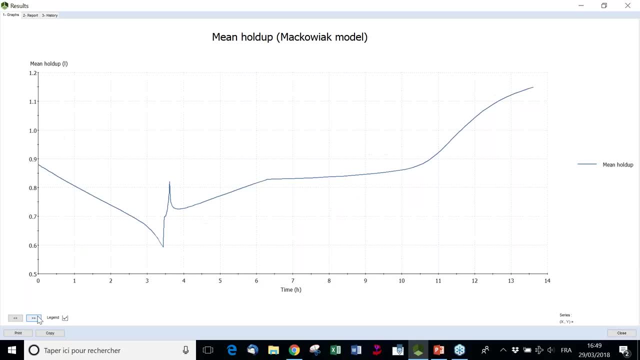 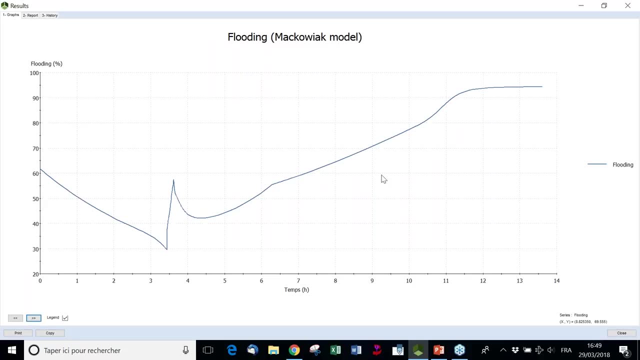 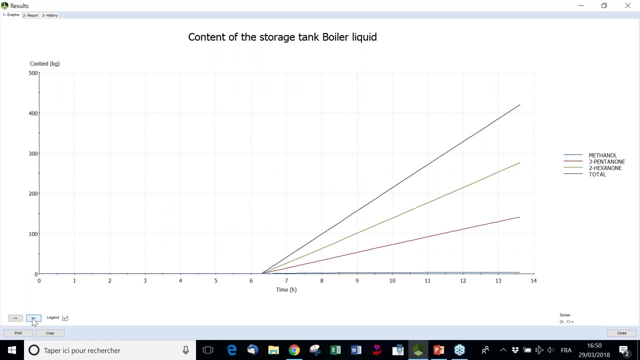 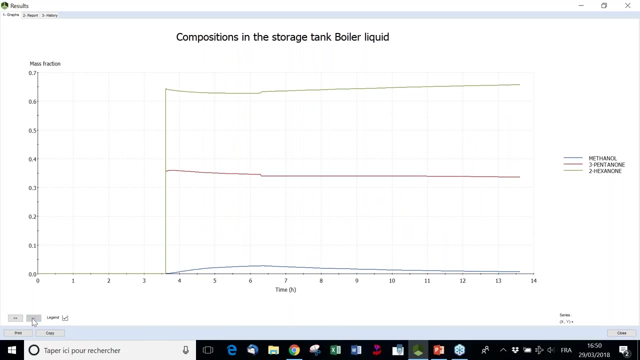 operating conditions and same. you have the holdup, which is calculated by the software, using the software and the corresponding fluid in and, of course, you have the contents in the storage tank at the distillate and also at the storage tank which is at the boiler. so 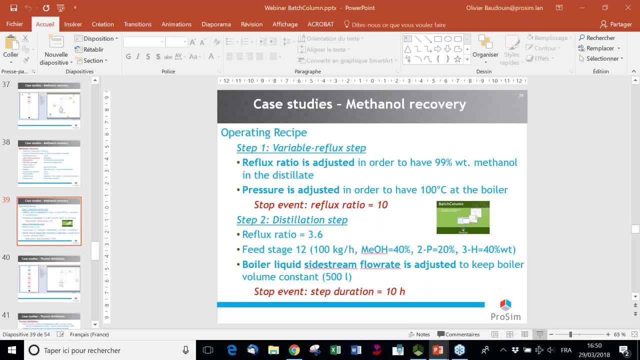 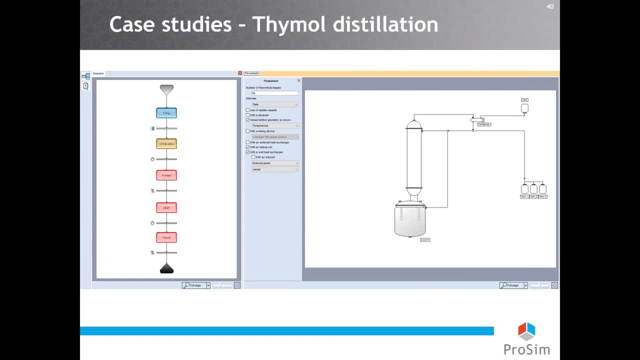 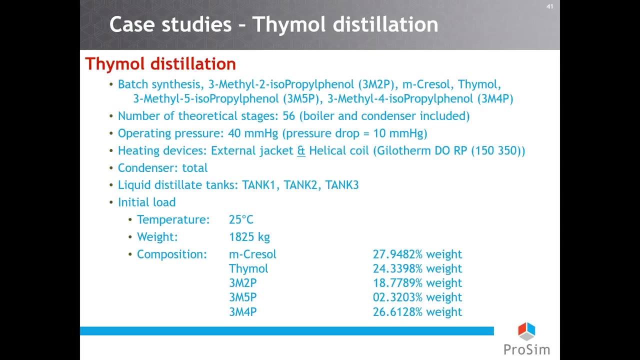 now let's go to the description of the next case. in that case this is for a team of installation, so it come back. it comes from a batch synthesis. there are five components which are included in the load at the end of the batch synthesis. the column has 56 theoretical stages, including the 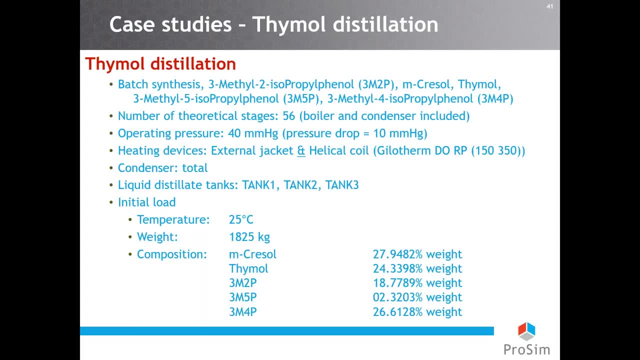 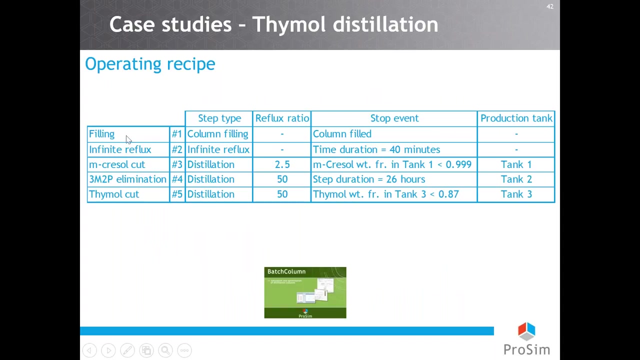 boiler and the condenser. it operates under the cool at 40 millimeter of mercury, and to his, in that case, jacket and analytical coil using the same. it's a transfer freedom and there are three correction tank and the initial load is this one. so the opening recipe is the first. we fill the column, then there is a infinite reflux step. 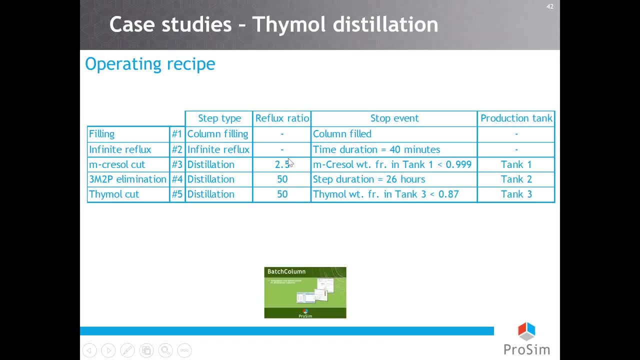 then a cut to recover the end crystal with a discharge or future issue equal to two. point five: this is the stop event, which is the weight fraction of end crystal in tank one. then we switch to the next step. the production will be sent. in tank two. we eliminate one of the 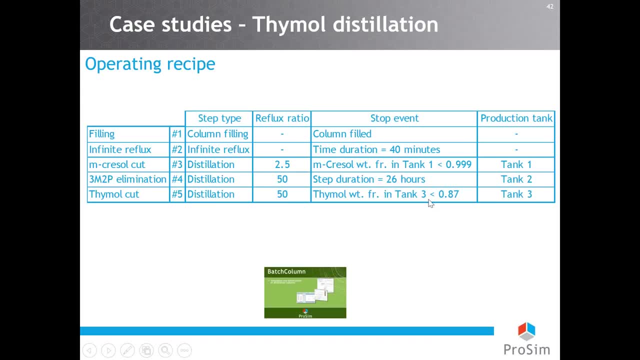 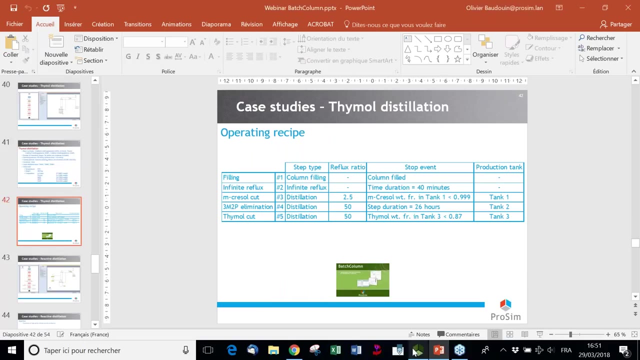 components. the duration is 26 hours and we switch to the next distillation step. we change the production tank and we want to recover Tmol with this weight fraction in that tank. we will want to recover it once we remove thextral thing in the mellanic Quick. 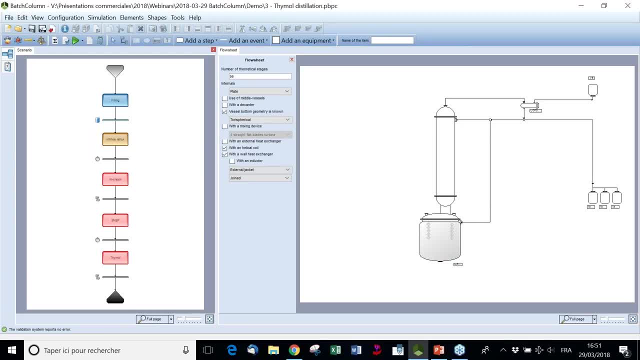 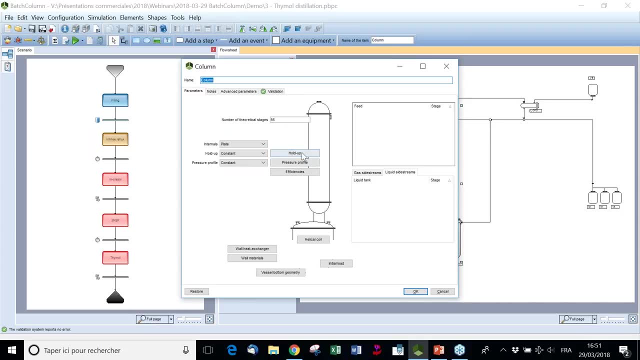 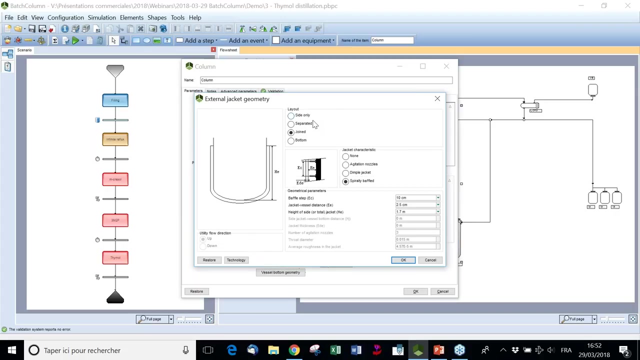 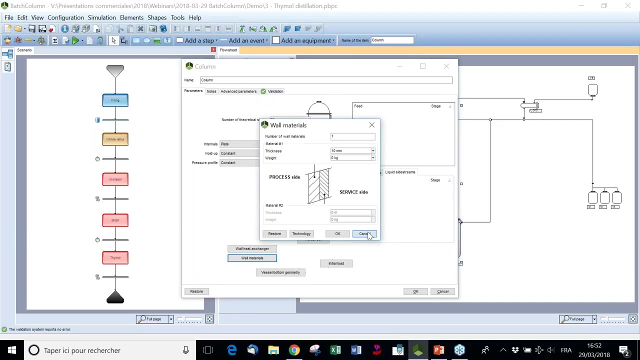 service fluid Academic Oval attacked today: 0, 10, 12, 12, 13, here with the corresponding parameters, and also the wall detection, which is an external jacket with these characteristics. the whole material is also described and, of course, the bottom geometry. okay, regarding the scenario: first a filling step, the event is automatic, then infinite. 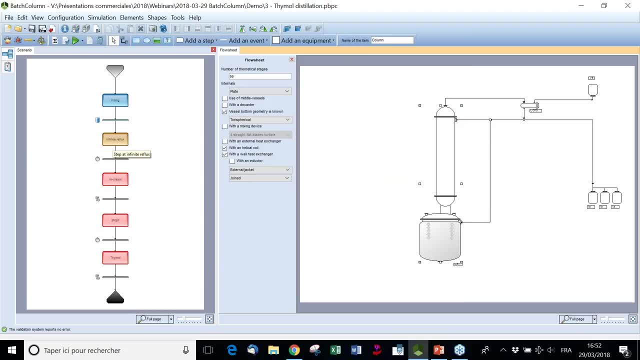 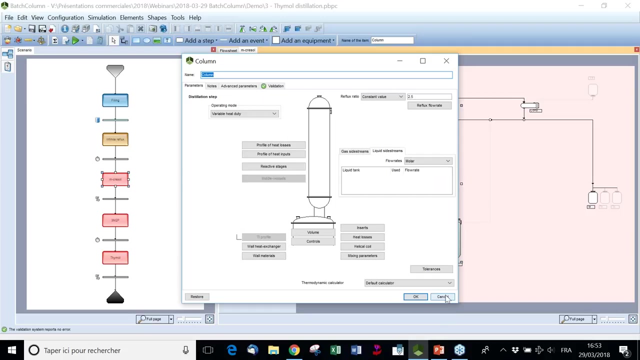 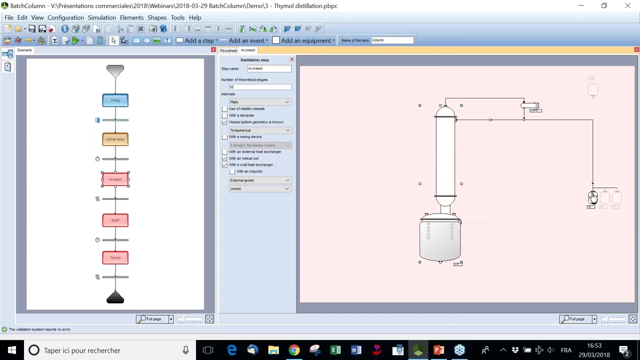 reflex and the heat duty of the boiler is of course calculated. we stop when the step is duration is equal to 40 minutes. then deceleration step. this decision step is performed with this reflex ratio. we stop when we reach the purity in tank one, which is the pollution tank, which is selected for the next step. we produce in the tank two. 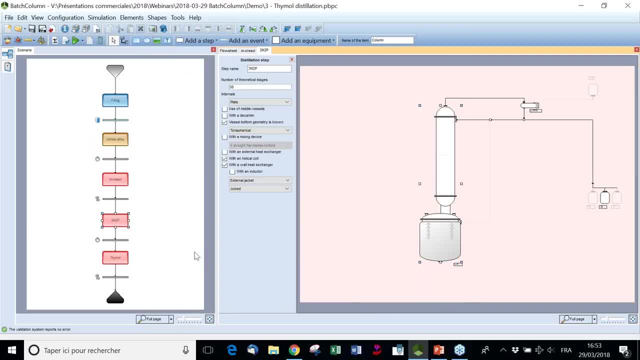 the reflux ratio is equal to 50.. then, after 26 hours, we will switch to the tmall production in tank 3 and we will finish when the event is equal to uh in the. the tmo weight fraction in the tank 3 is equal to 0.87. 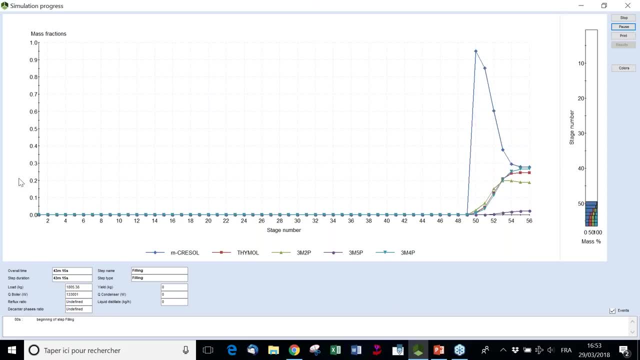 so here you have the boiler. still here, this is the condenser, and you can see the components which are filling, step by step, the column in this example. what is important to note is that we can use more than just one uh heating device in fact. so how we divide this into the camp. so they are really small, apparently. 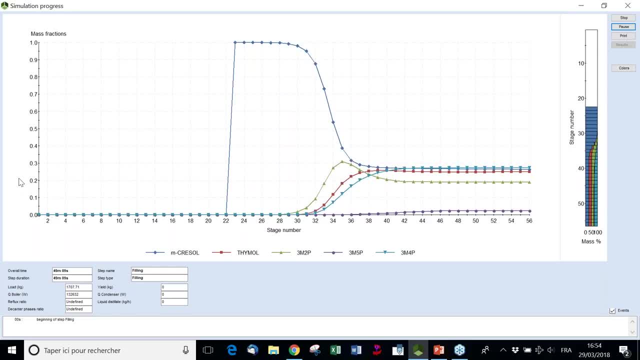 so we can Conventionally think that these are cold from the. uh, these customer safe TV lead. filling of the column. you have more than 50 minutes to fill this column. here you have the heat duty of the boiler, which is calculated given the characteristics we have provided for the for both of the. 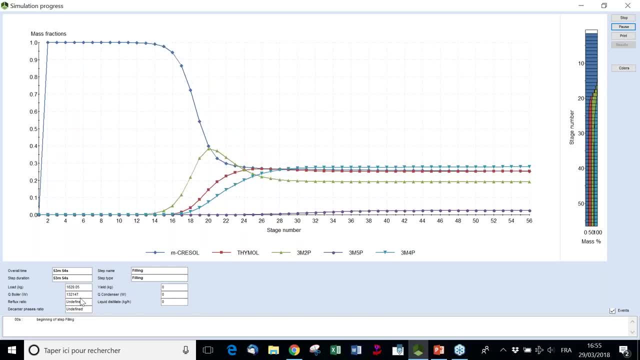 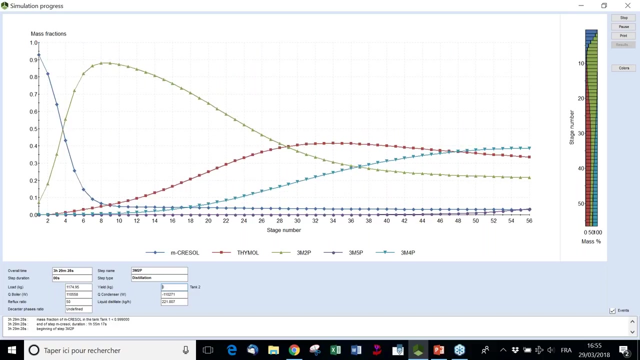 uh mixing heat, heat transfer equipment, and then the distillation with the infinite reflux in order to classify the column, and then we have a distillation with this reflux ratio. here you have the evolution of the distillates: the which is recovered, tank one- then the evolution of tank two. 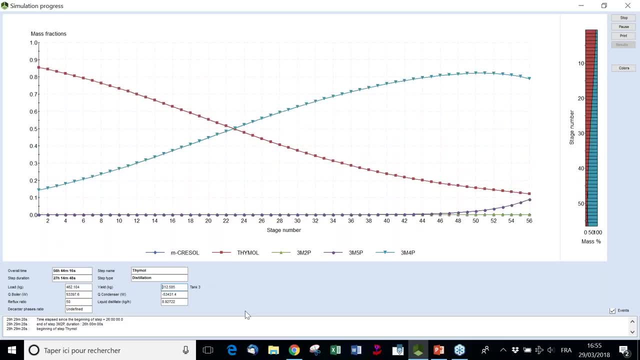 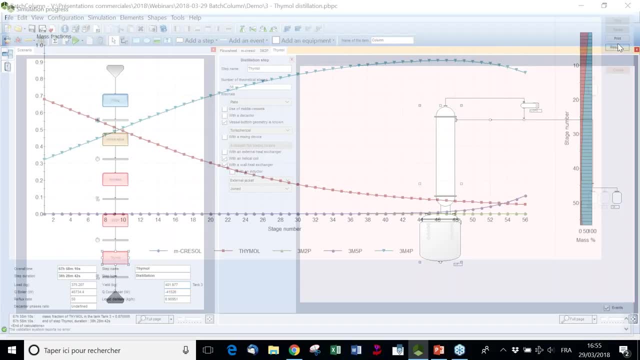 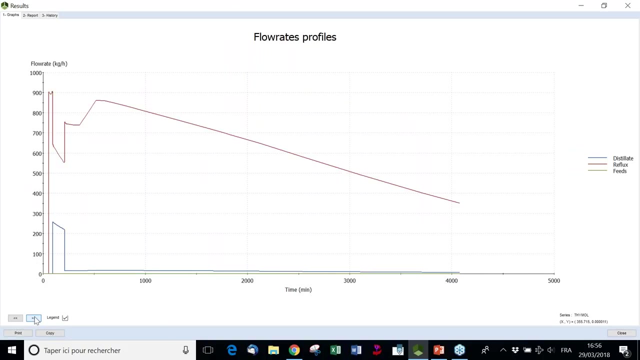 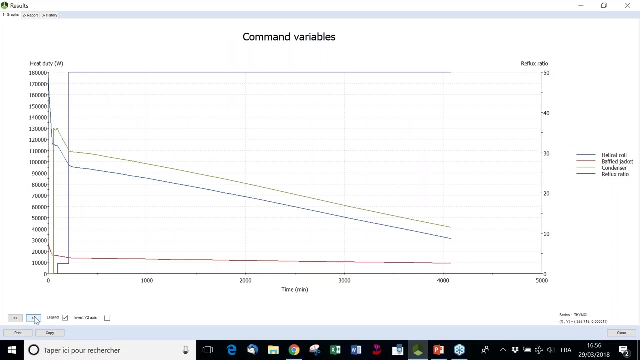 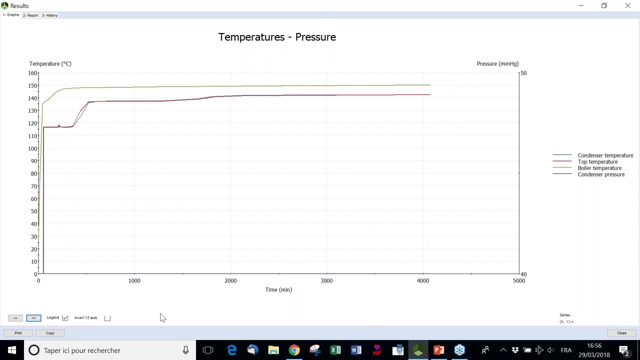 and the tumor recovery. so for the results, same. we have the mass fraction, distillate, mass fraction in the boiler and the evolution of the flow rates for the, for the distillate and the reflux, and the duty at the condenser and at the boiler. here you have the evolution of the pressure profiles. 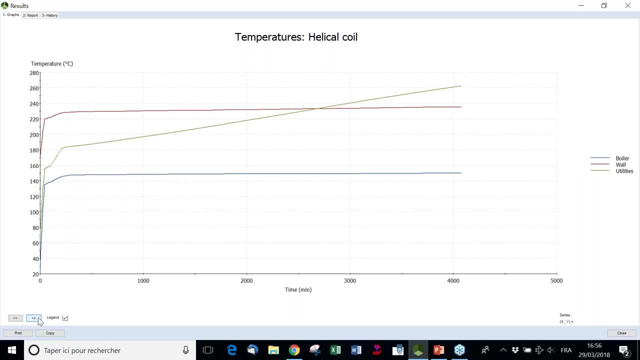 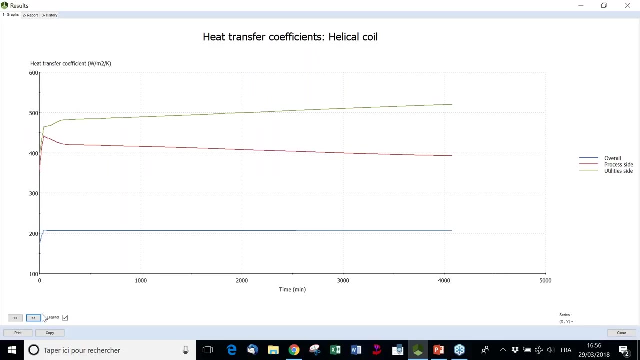 and the. what is important is this is the information about the heating devices. for the helical coil you have the temperature of the wall of the, the boiler and of the utility, and here you have information about the heat transfer, and same for the. here you have the. 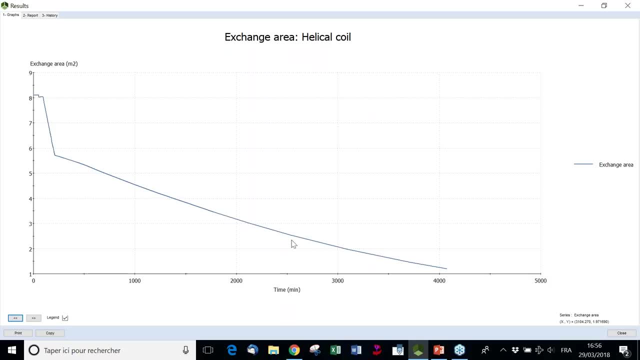 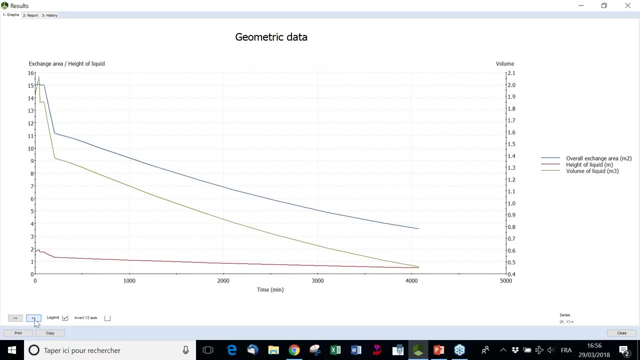 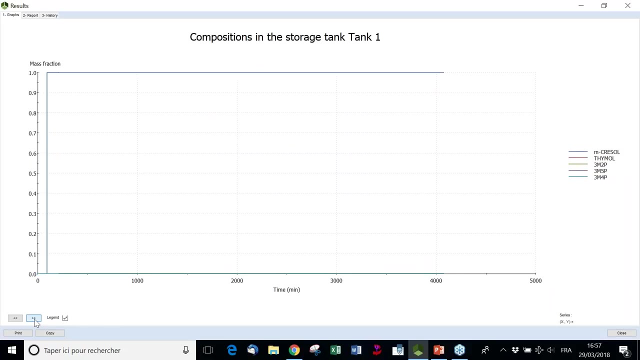 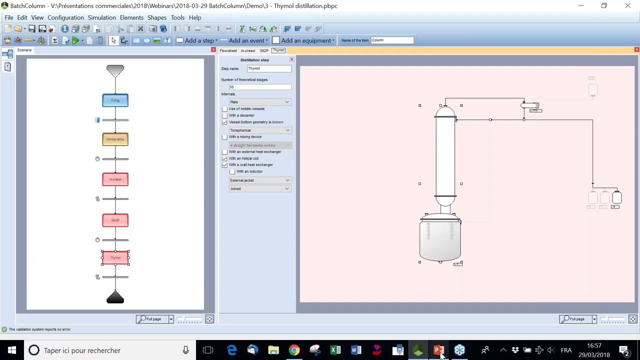 evolution of the heat exchange area, which is not the same during the simulation, and same for the bathroom jacket. the physical properties are also calculated and so on, and of course the the storage contents of tank one, two and the three which is containing the tummel. so now we can go to the last example, which is a rated distillation. 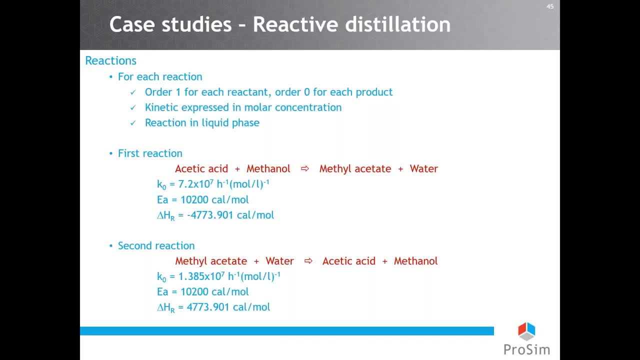 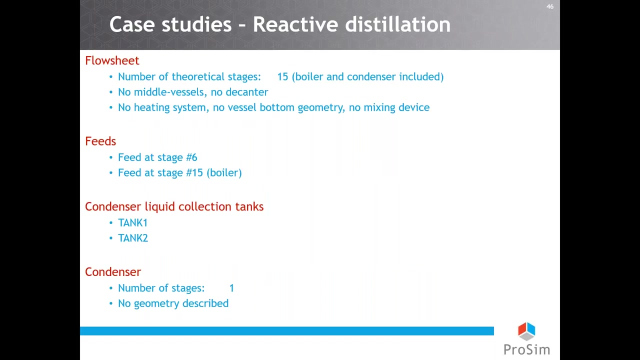 so there are two reactions described by uh, a, re, new, slow. the first is the volatile distillation. The second one is the reverse of the first reaction. There are 15 chemical stages. There are two feeds also, one at the stage six and the other at the boiler two collection tank. 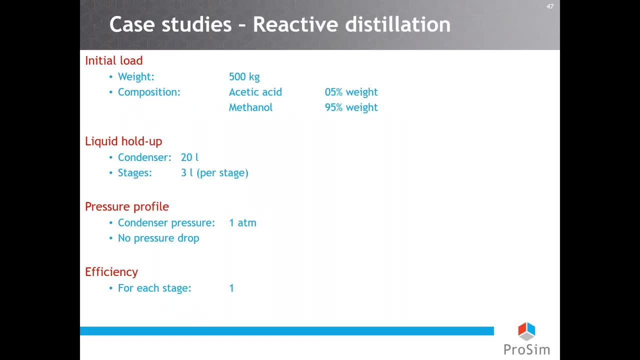 We have one stage at the condenser. The initial load is 500 kilograms- mainly methanol, And the liquid holder for the condenser is 20 liters And for all stages we have three liter. We are operating at atmospheric pressure. 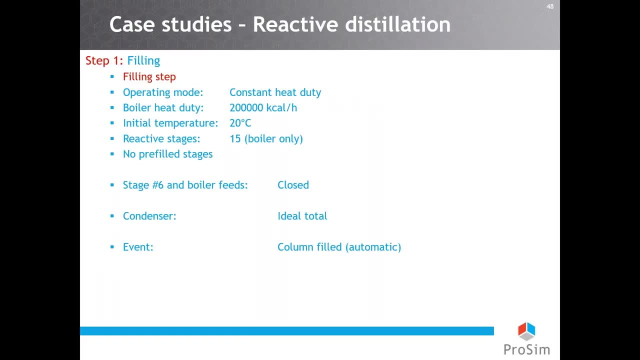 First step- this is a filling step- with this information. During the distillation, we have a reflux ratio which is equal to three, The boiler feed is open, We feed pure acetic acid, The production tank is tank one And the event is the methyl acetate mass fraction. 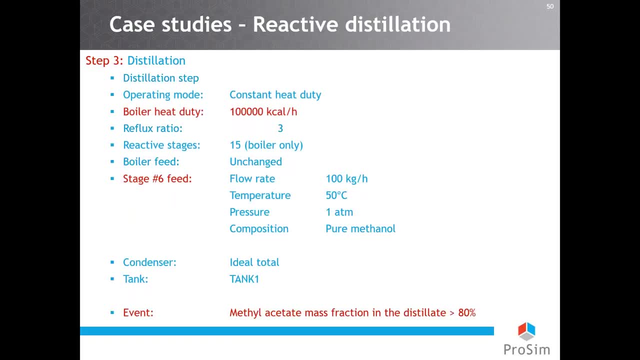 in distillate. Step three: We change the heat duty at the boiler, We open the feed at stage six, which is pure methanol, And we produce still in tank one And the event is the methyl acetate mass fraction in the distillate. 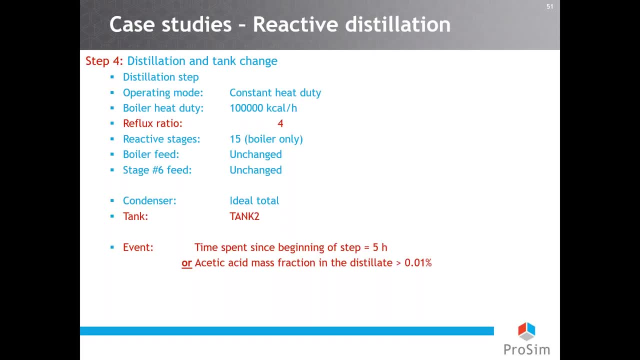 For the step four, the reflux ratio is changing to four, The production is sent to tank two And we have two events which can be reached. The first one is time duration For the step And the second one is the acetic acid mass fraction. 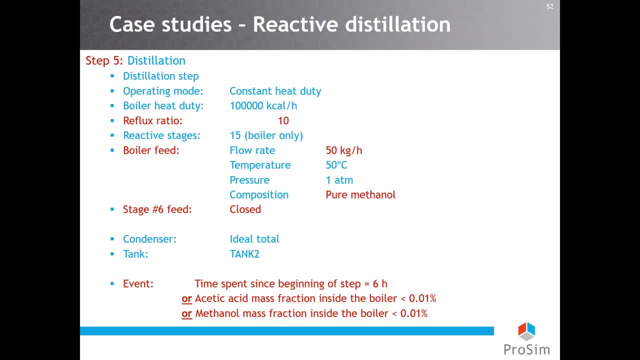 in distillate, The step five, you have the reflux ratio which is equal to 10.. The boiler feed is changing. We close the feed at stage six And we have three different events which can be reached: time duration or acetic mass fraction in the boiler. 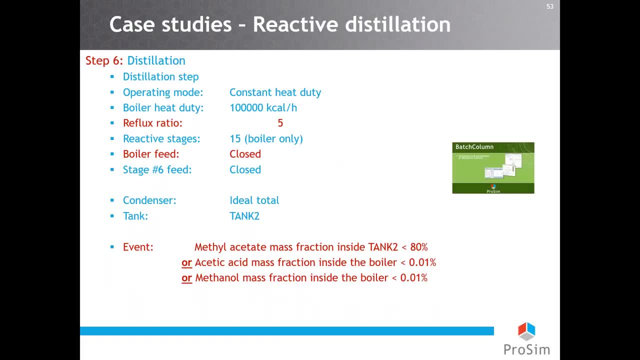 or methanol. mass fraction in the boiler. And the last step: we change the reflux ratio. There is no more feed And the stop events are: mass fraction in tank two for the methyl acetate or acetic acid. mass fraction in the boiler. 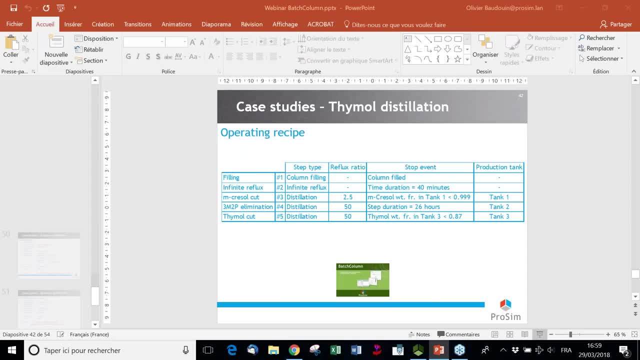 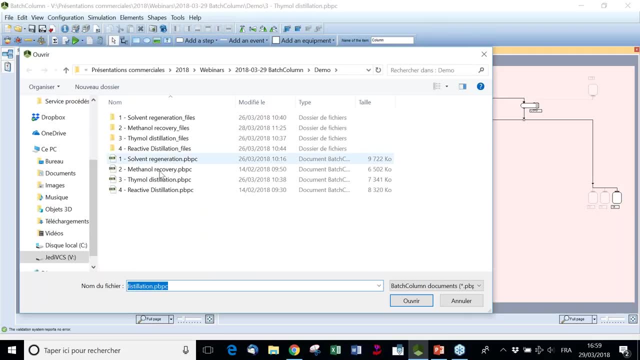 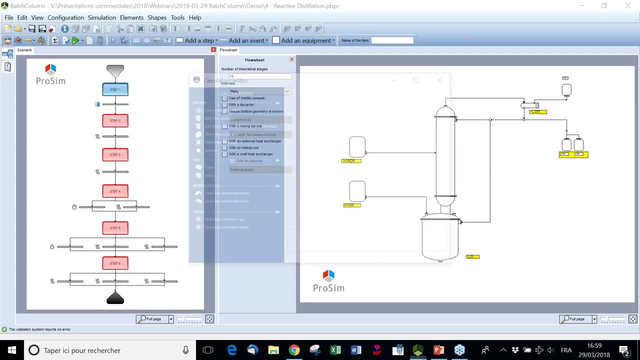 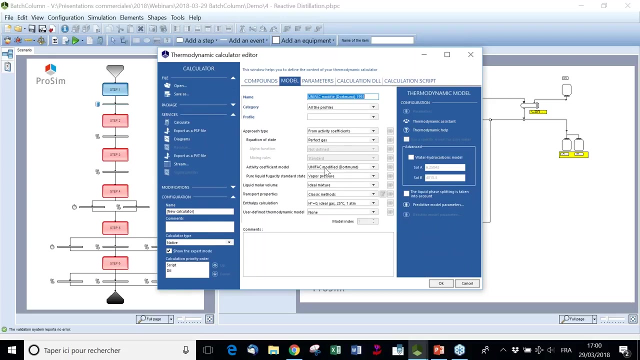 or methanol mass fraction in the boiler. So let's go to the example. So in that case We can go to the thermal description, because we will use a predictive model which is UNIFAC, And in that case, what you can see, 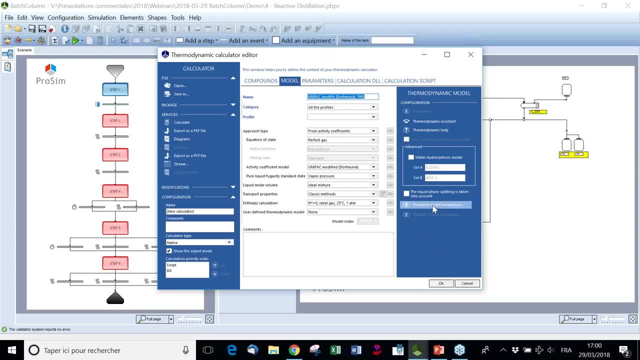 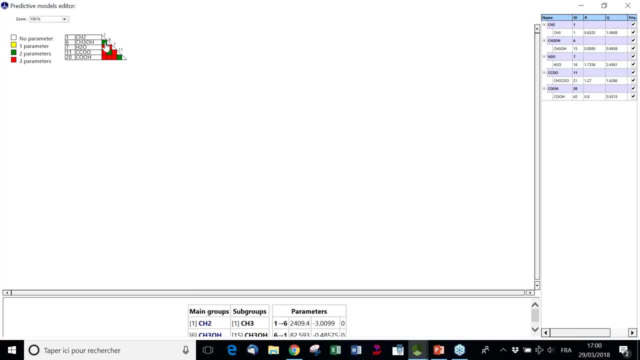 is that you have the predictive model parameters, And so you will have access to information about group concretion methods for the mixture you have described in the calculator. That means which groups are involved, which are the parameters- group interaction parameters- and what are the characteristics. 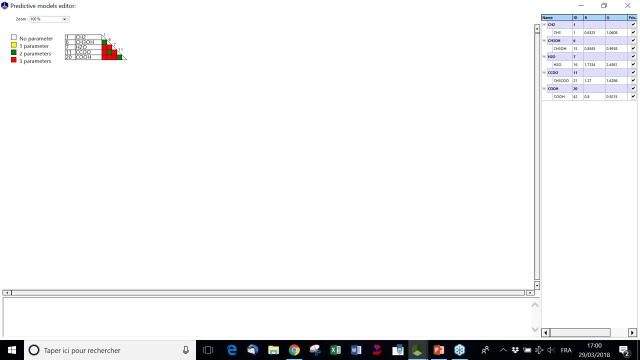 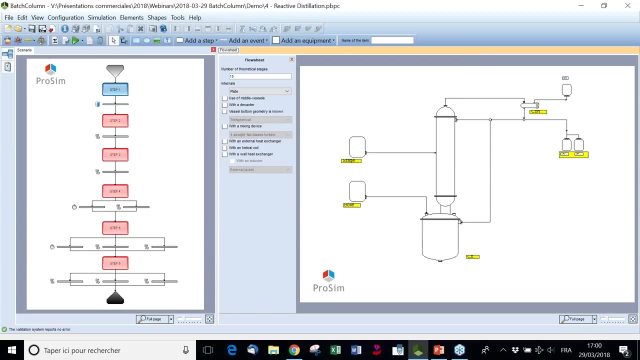 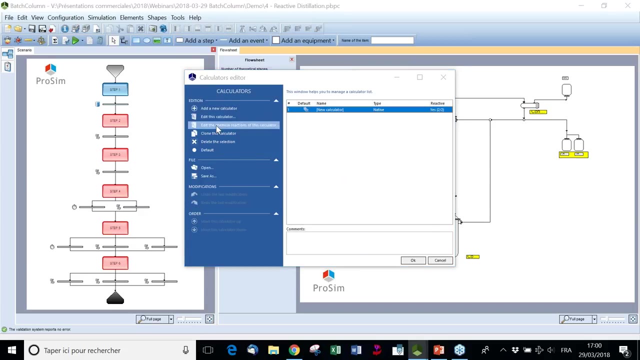 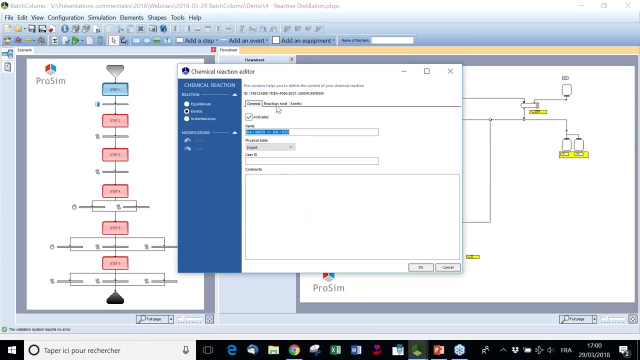 van der Waals and the volume and the surface area for this model. Sorry, Here we will go to the description of the reactions. So we select the kinetic model. We can provide the reaction heat or it can be calculated from the standard. 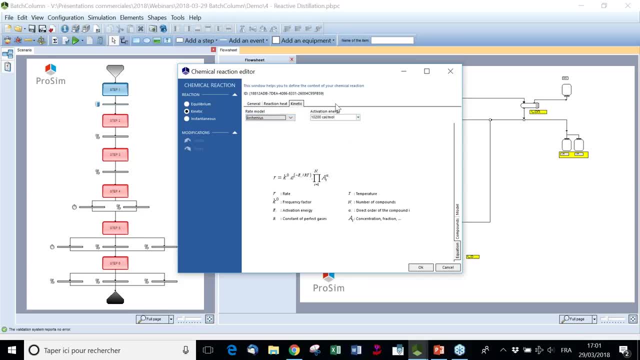 And here for the kinetic, we select the Arrhenius model, We provide the activation energy. For the compounds, we provide the stoichiometry Negative: if it's a positive, it's a product. Negative is a component. Negative is a component. 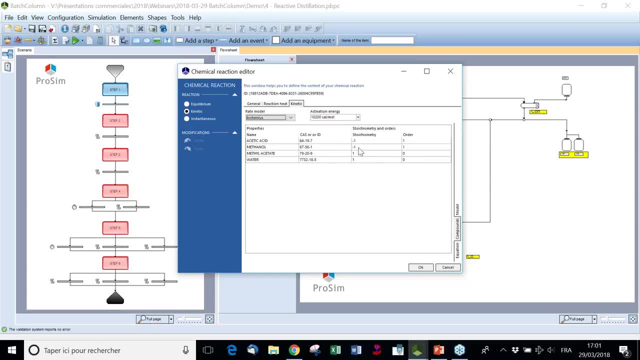 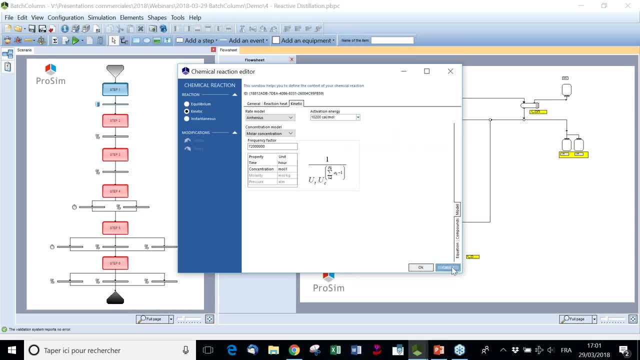 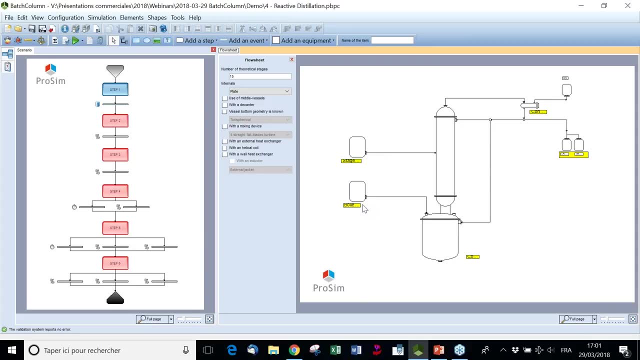 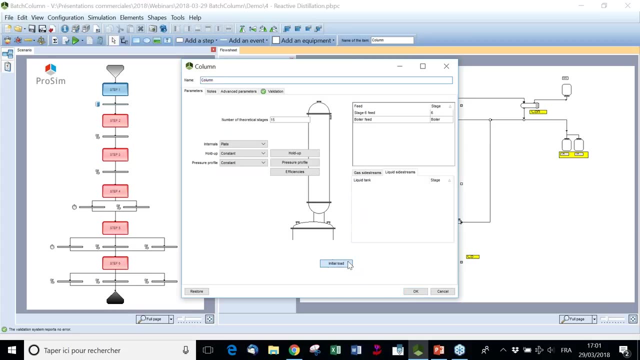 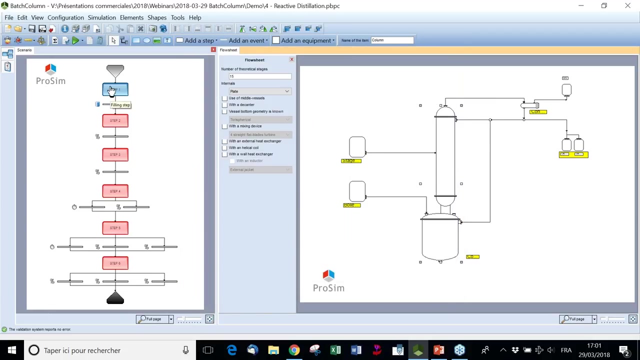 the frequency factor which is used, Of course, same for the second one. And then here we describe two feeds, two production tank. Here we provide the initial load, And then we start for this with the filling step, And here we describe the scenario. 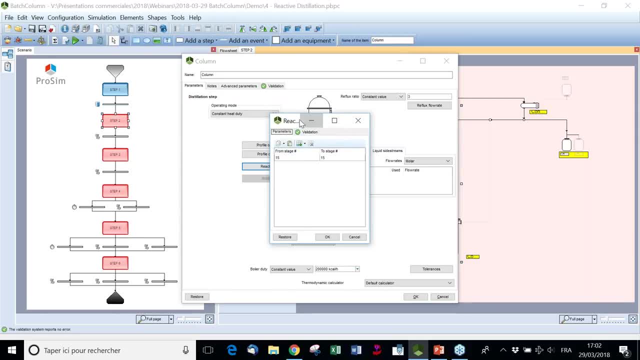 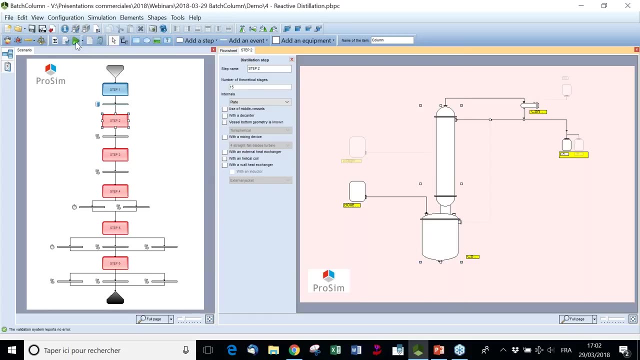 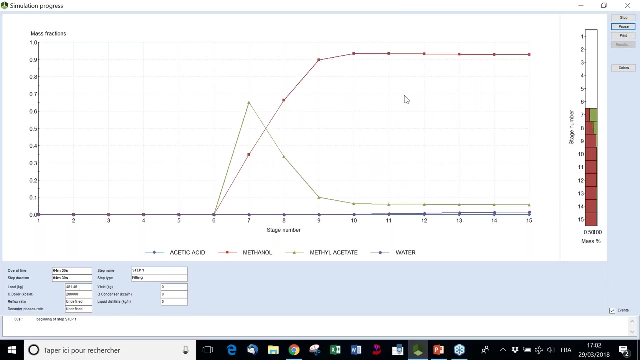 For each step we describe, which is the reactive stages. In that case, only the boiler is reactive, And so we can run. We can run the simulation. It's only a little time. When the boiler is activated, we do the final work. 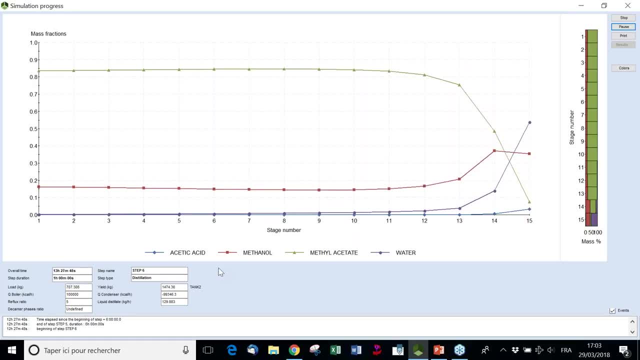 So you can see There are two phase of the linear design. So you can see this one. You can see the layout. This one is the vertical layout And then you can see the direction, And this one is the lateral layout. 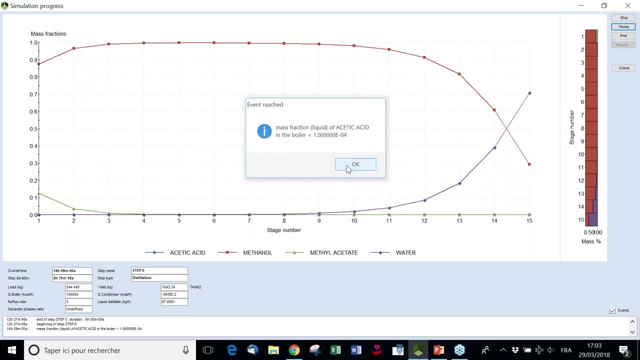 And this one is the horizontal one. You can see that the clarity, You can see that the range is greater, You can see that the Ship and Class are more in the middle. The philosophy is, as I said, the velocity is more greater. 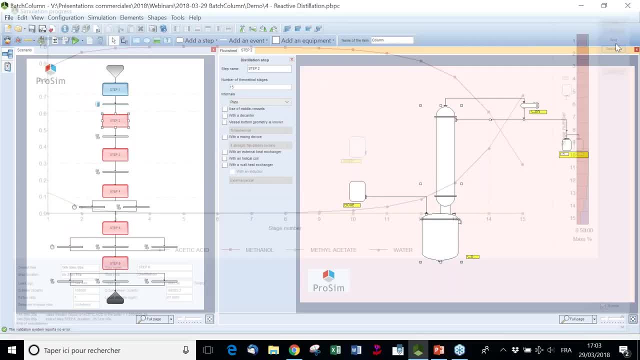 You can see we are load longer. We can see the time- This is when we can use the difference between speed and velocity- And then we can see the mass friction in distillate. And then we can see the mass friction in distillate. 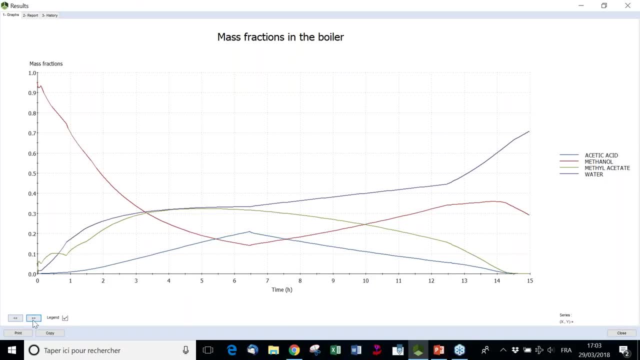 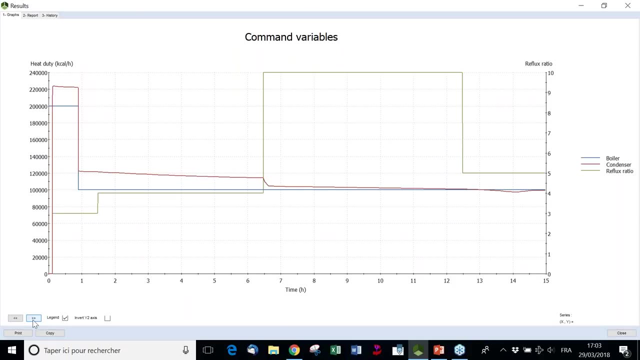 distillate, same for the mass fraction in the boiler, and you have information about fluoride also and so on. so with these four examples I can I see that I think that we show you some of features of batch column. of course, one hour is very short, so if you have, if you want to see more about batch column, well, thank, 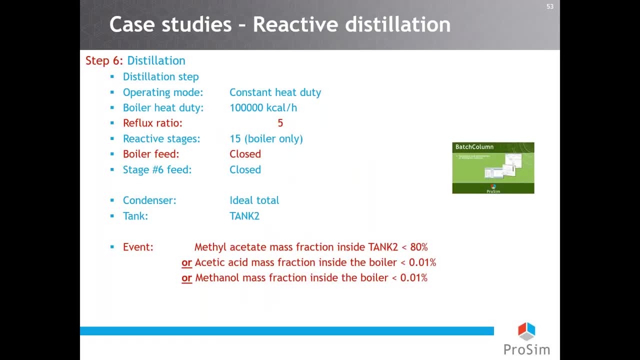 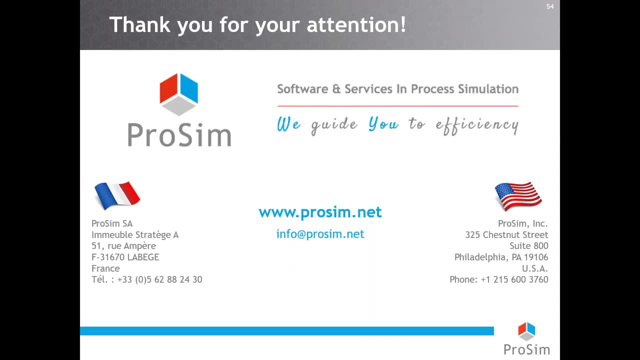 you, Olivier, for for this presentation and thank you all of you for being here with us and for bearing with us for this webinar. please take the time the to answer the questionnaire to let us know if it makes your expectations. please take the time to answer the questionnaire to let us know if it makes your expectations. 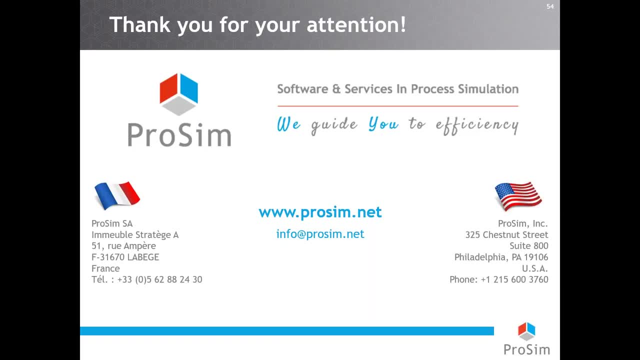 it's only four questions that will be prompted after we have. a replay of the webinar will be sent to you in a few days and obviously, we remain at your disposal to collaborate on your simulation and optimization project and don't hesitate to contact us. so bye, everyone, and thank you very much. you.